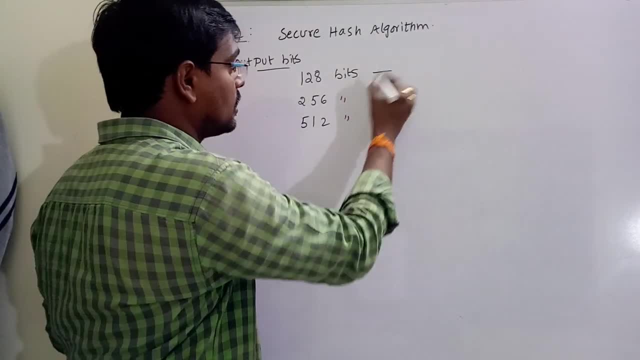 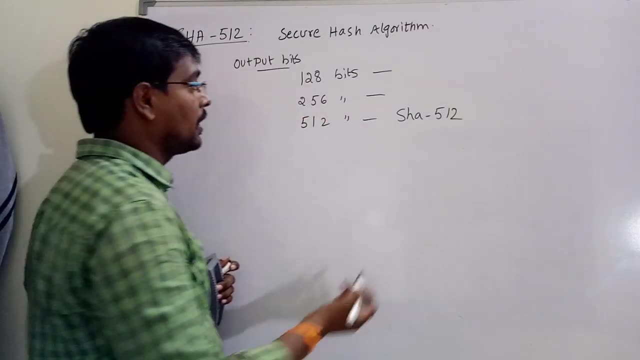 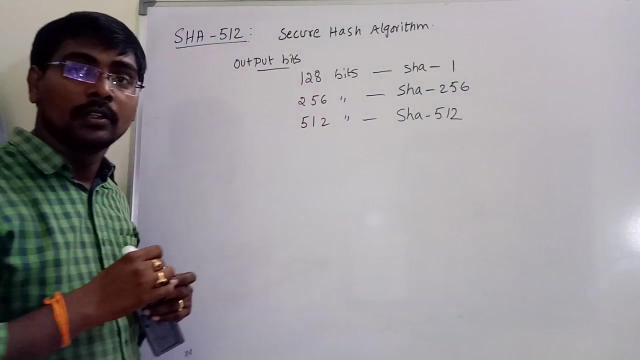 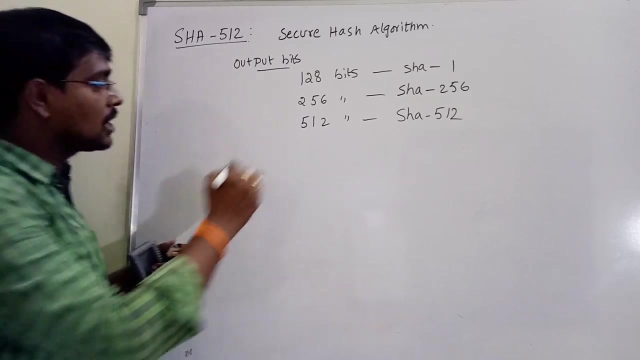 depending on outputs, this is called sha512. if it is a 512, this is called sha512. this is called sha 256 and this one is called sha1. so, depending on number of output bits, we are dividing the names, so we will discuss sha 512. that is the number of output bits in this example. 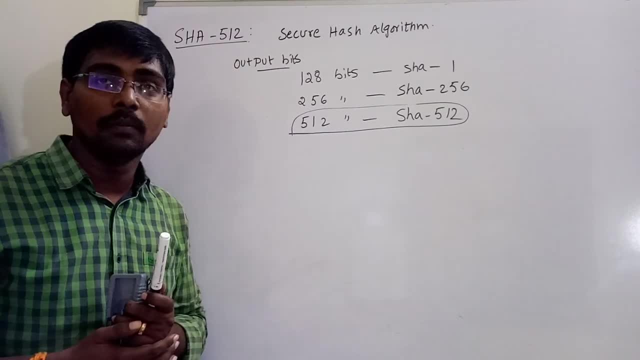 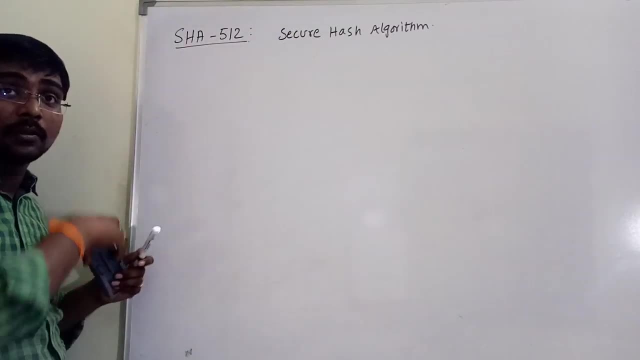 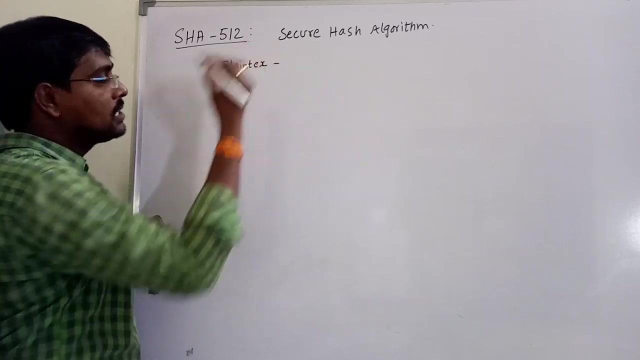 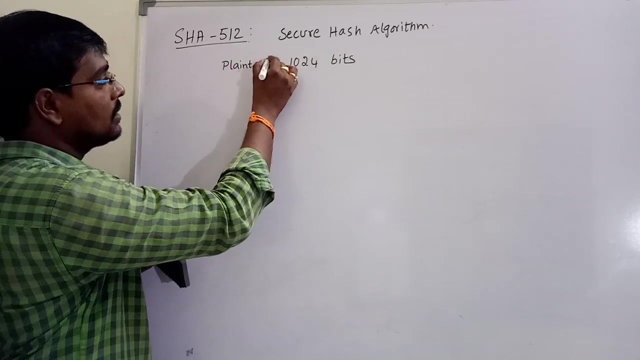 is, that is in this algorithm is 512 bits. okay, now we will discuss what is the sha algorithm and why, how to implement this algorithm, before going. the plain text: What is the size of plain text? The size of plain text is 1024 bits. Remember, here, not the size of plain text, Here the size of plain text. block The 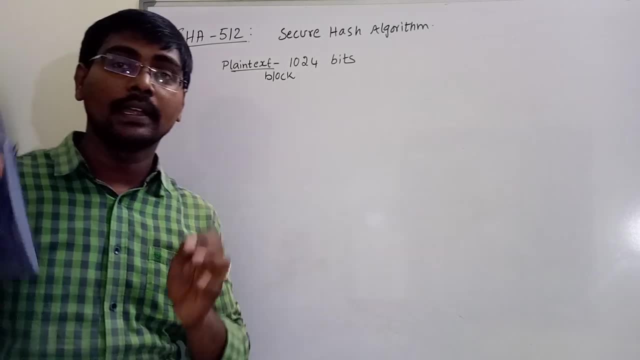 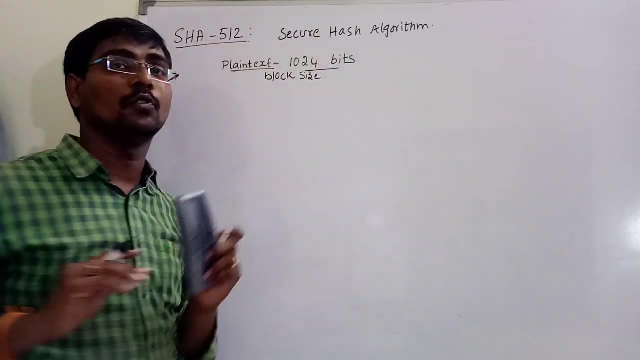 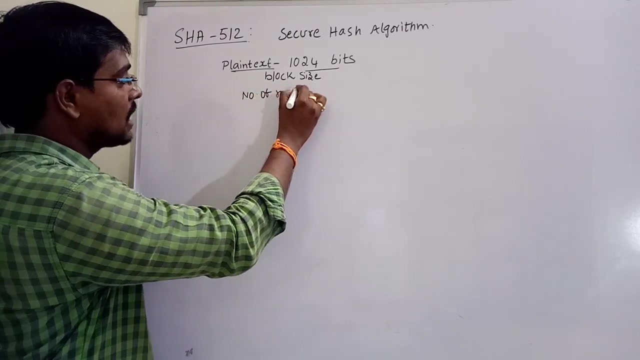 size of plain text block. that is, the entire plain text is divided into different number of blocks. Each block size is 1024 bits, Each block size is 1024 bits And number of rounds in this sharp 5-hole algorithm is 80. So first one is the plain text block size and the number. 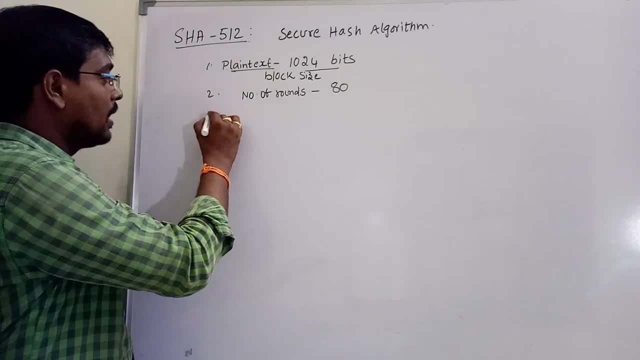 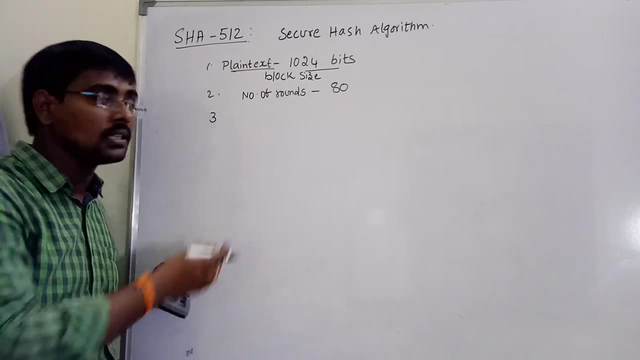 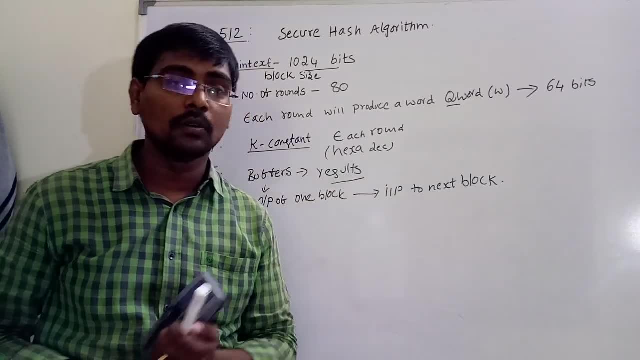 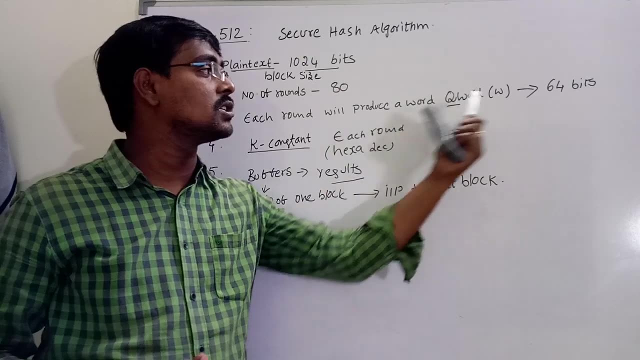 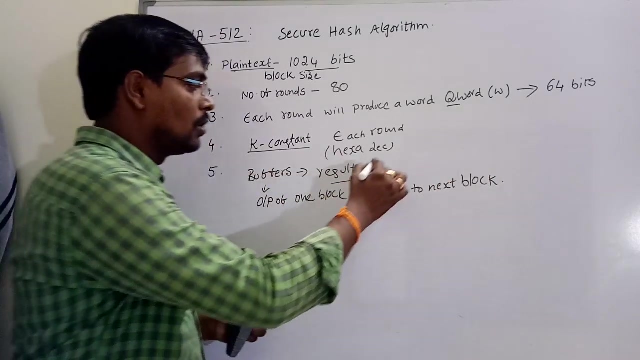 required. What is the size of output? Size of output is 512 bits Each buffer. each buffer size is 64 bits, So total 512 and buffer size is 64. So 64 into H. So we need 8 buffers. 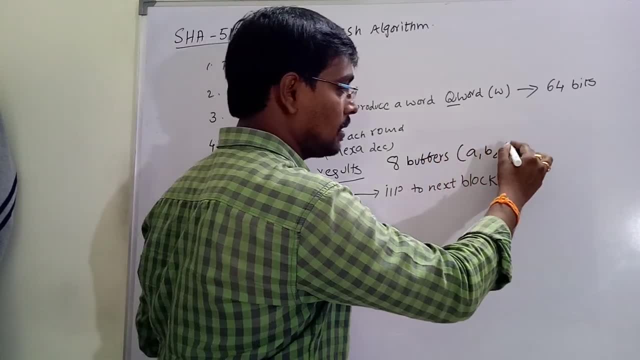 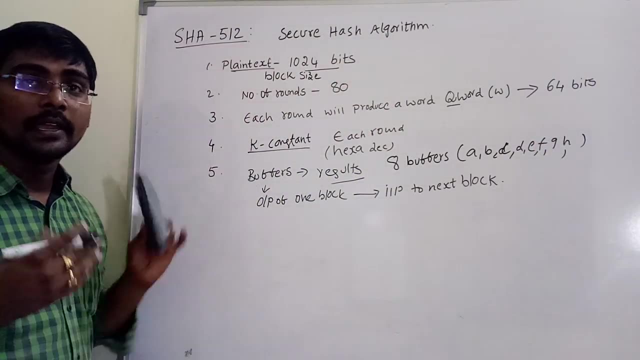 And the names of buffers are A, B, C, D, E, F, G, H. These are the 8 buffers used in our program, 8 buffers used in our program. So this is clear, This is clear. Now we will. 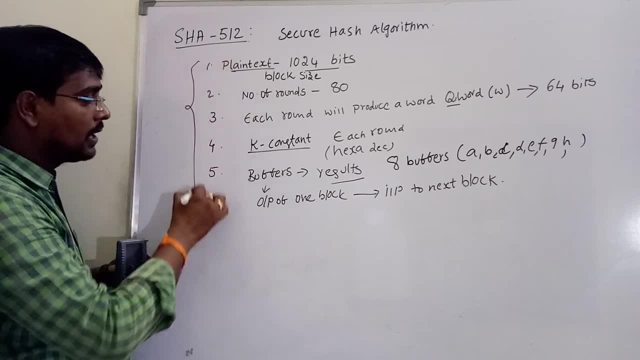 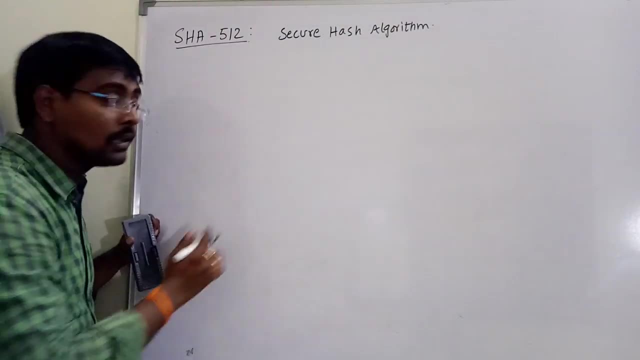 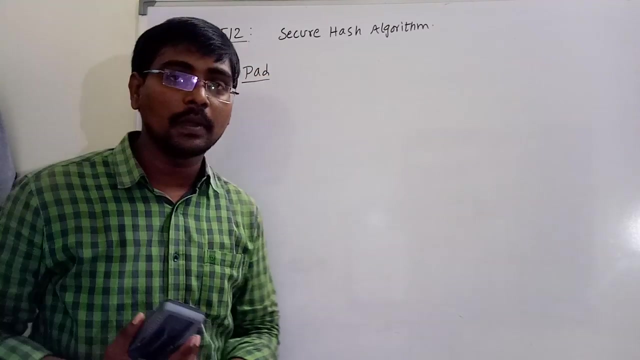 move to the algorithm. So after identifying all these, so I reference one- What is the step procedure? Procedure is padding On most all algorithms. the first step is padding Here. what is padding Means? we are taking the input Here. size of each block is 1024. 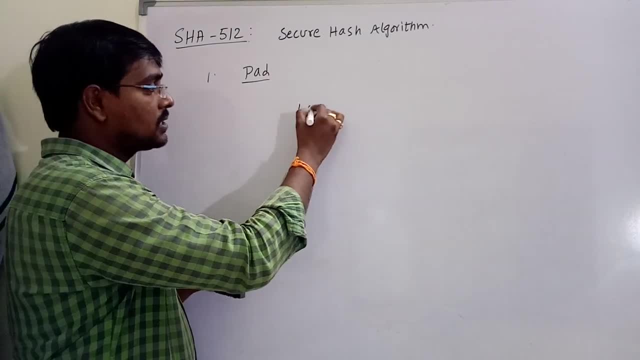 bits. For example, if my algorithm is 1024 bits, then I am taking the input. So I am taking the input. So if my plane test size is 1025, if my plane test size is 1024,, what? 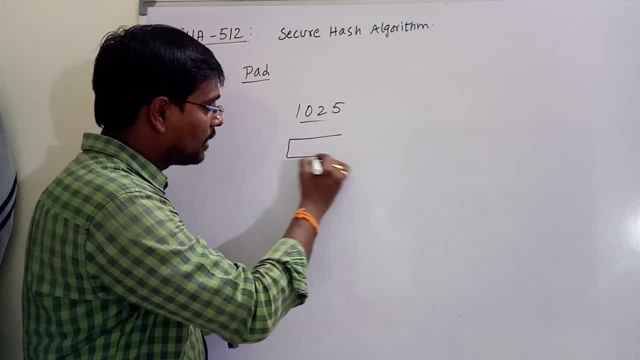 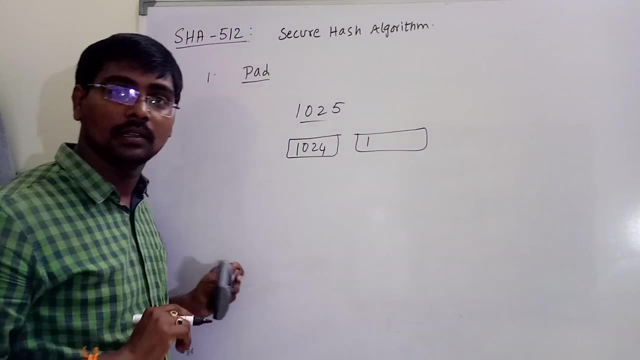 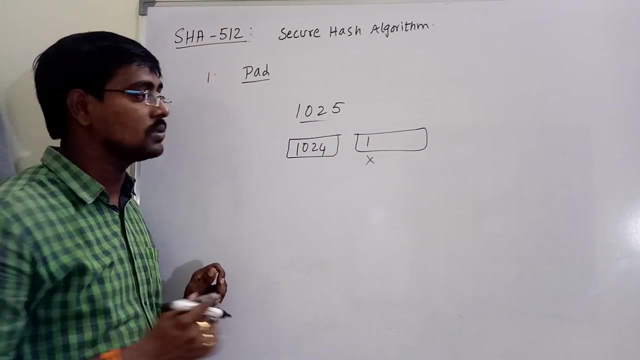 we will do. I am dividing the plane test of one block of size 1024 and another block of size only 1 bit, But it is invalid. in this algorithm. Each block necessarily definitely contains 1024 bits, So I am padding these 1023 bits. So what is our first step? Our? 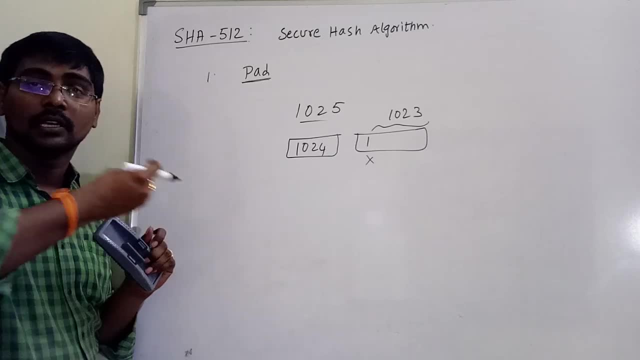 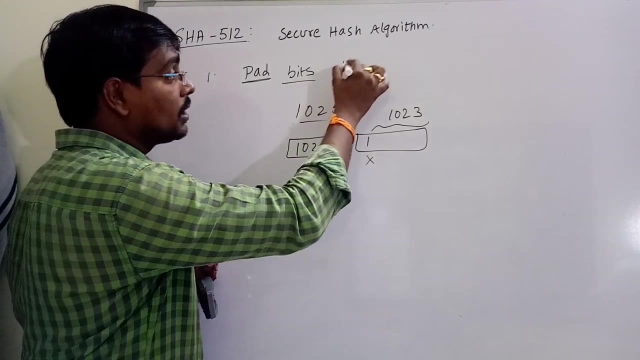 step is padding. First step is padding of the plane test. So padding the bits, Pad the bits. So what is the condition? Pad the bits with remember, 100 and so on, Starting with 1 and 0. Suppose. 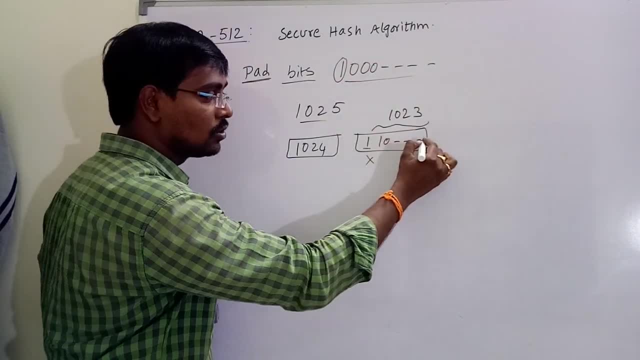 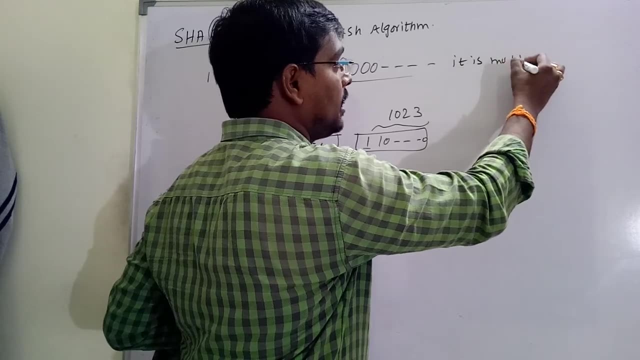 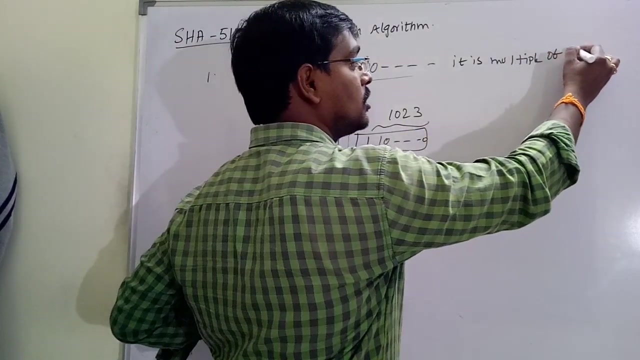 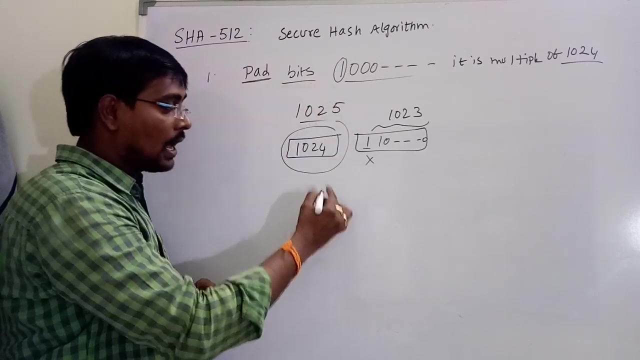 this is our bit 1000 and so on, Padding the bits such that it is multiple of 1024.. Multiple of 1024. That means, if our number is suppose our test size is 1025 bits, I am padding the. 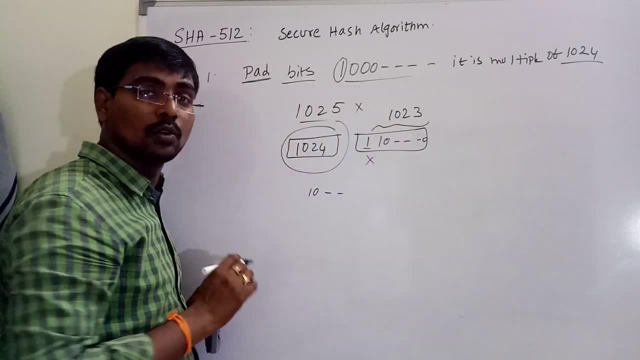 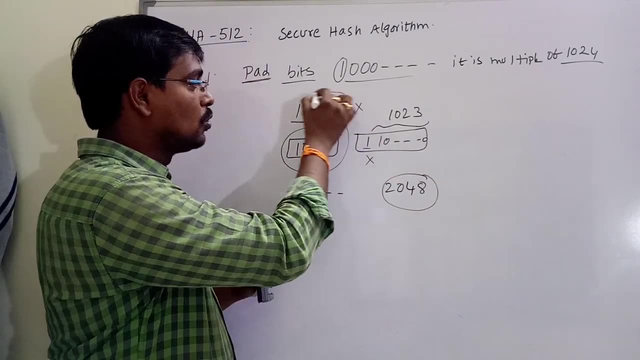 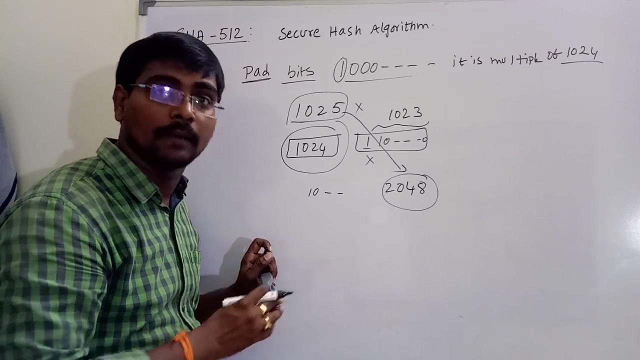 bits, Such that it is multiple of 1024 means 1024 into 2.. Suppose 2048.. This 1025 bits is converted into 2048 bits. And at the time of padding- remember at the time of padding- leave last 120 bits. So we have to keep the 1024 bits. We have to keep the 1025 bits. We have to keep the 1024 bits. We have to keep the 1024 bits, We have to keep the 1024 bits. 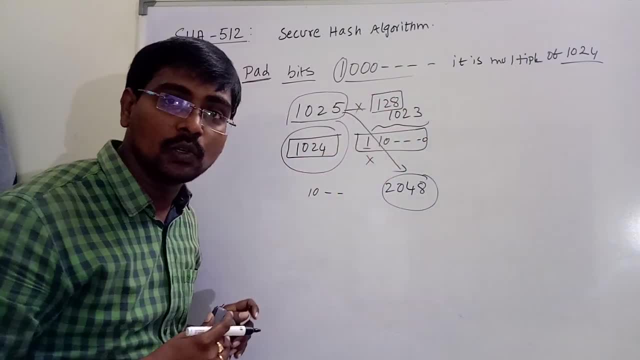 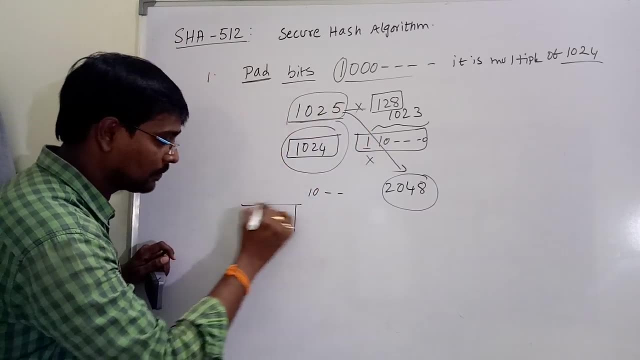 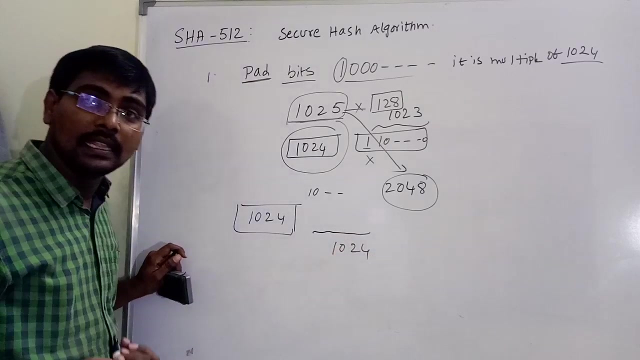 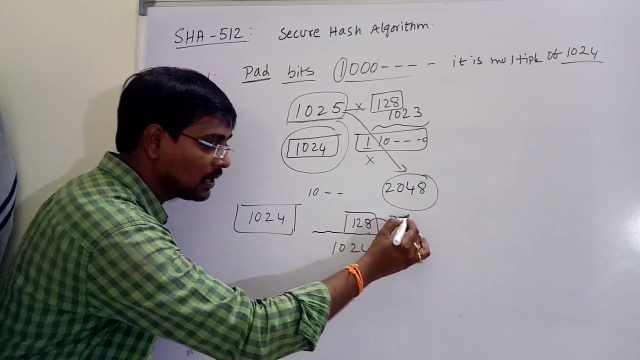 128 bits. Leave last 128 bits. that means, suppose This is our number. 1024 is added. 1024 is added next to how many numbers? 1024 in this 1024 number For that 128 bits. this 128 bits is plain test. I am adding only these bits. 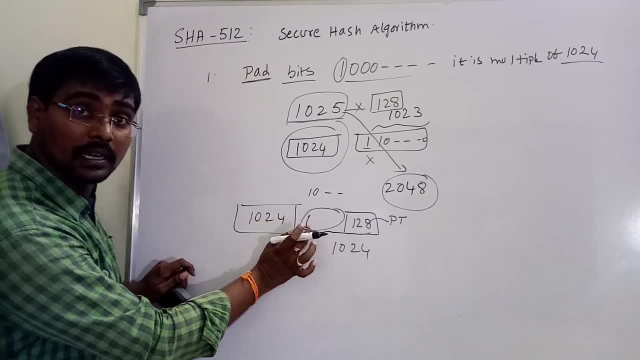 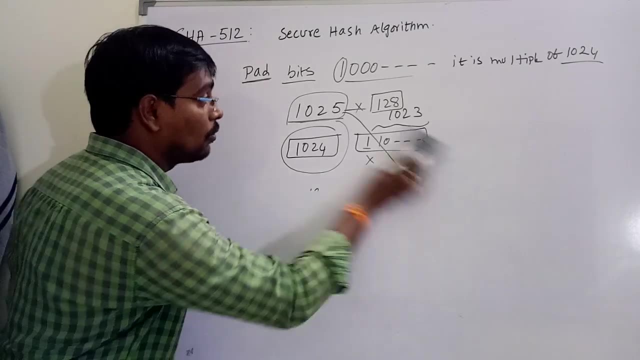 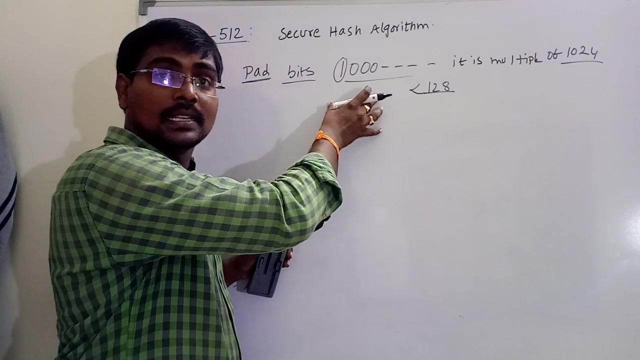 For example, this is the remaining bit at this position, one. I am adding only this. That means how we pad the bits, we padding the grid such that it is less than 128. It is less than 128 multiples of 1024 in second step add: 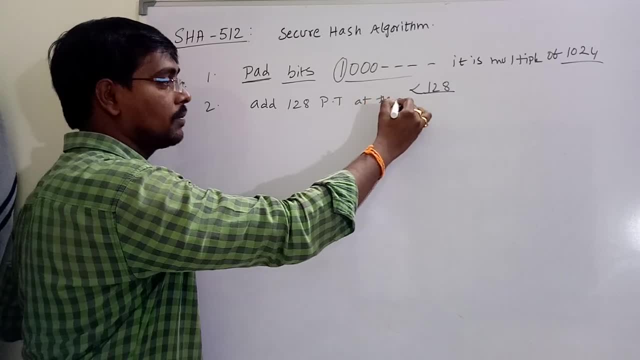 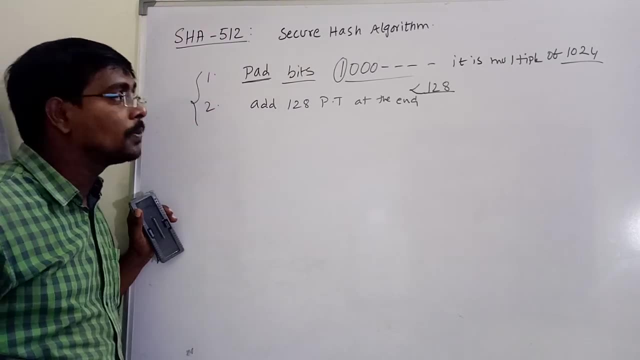 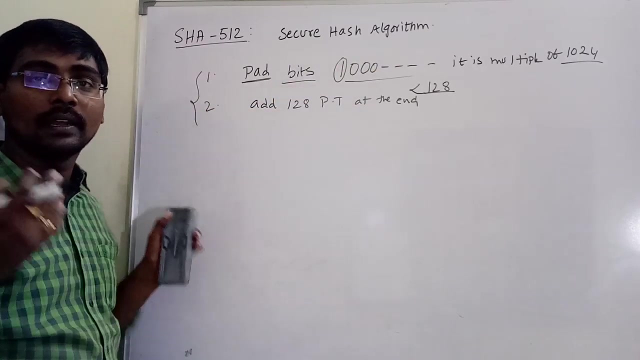 128 plain test at the end, 128 bit plain test at the end. That means by combining step 1 and step 2, We are getting a plain test, or which is multiple of 1024. We are getting a plain test which is a multiple of 1024, and remaining algorithm is very simple. remaining one is use. 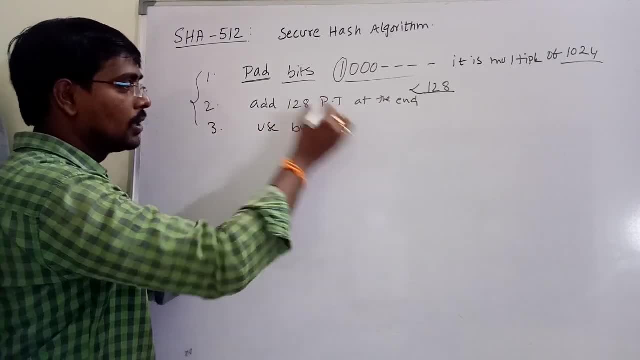 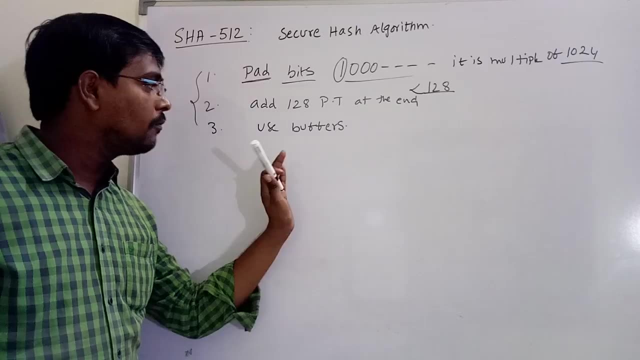 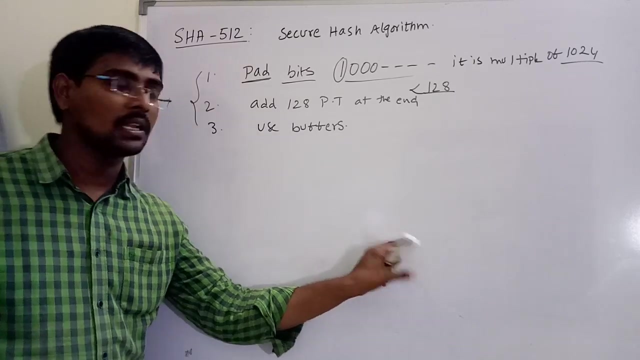 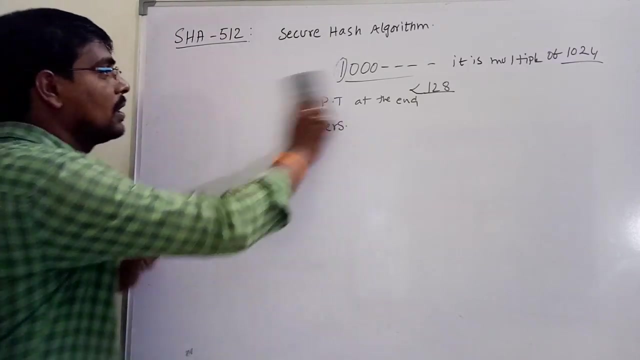 buffers. Use buffers and perform operation on each block and each row. after completion of one row, that result is the transfer to next row. so total: complete all the 80 rows. after completion of 80 rows, Results is the transfer to the next block. so we will show this was a diagram- by understanding the diagram. 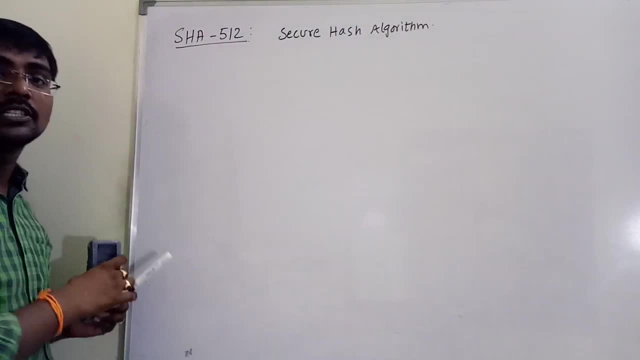 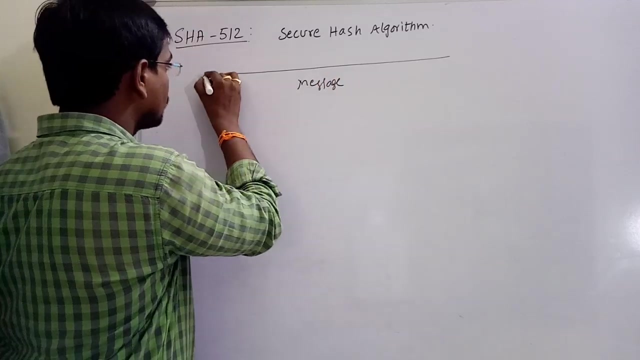 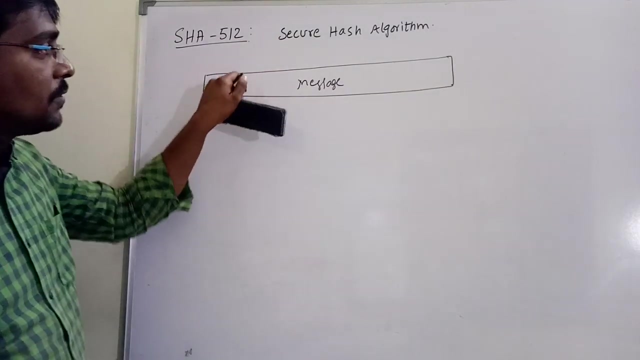 It is very clear. the shawl garden is very simple. What is the diagram? first, I am getting a playing test, for example, If my message is young. So This is the message, the. in this message i am padding some bits, suppose. if it is not multiple of 1024 bits, if it is not. 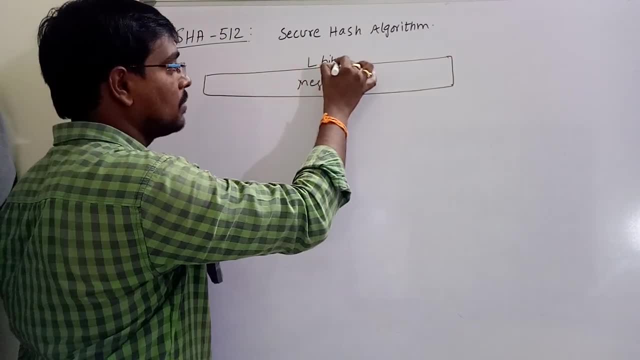 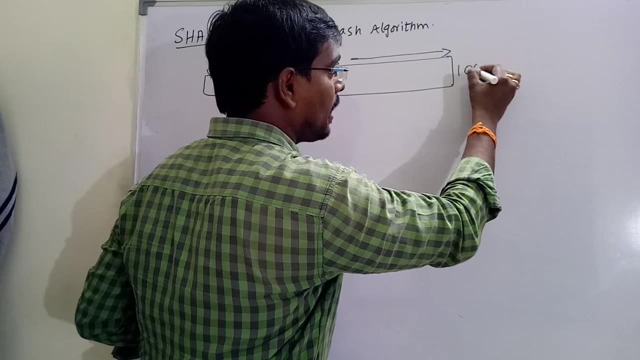 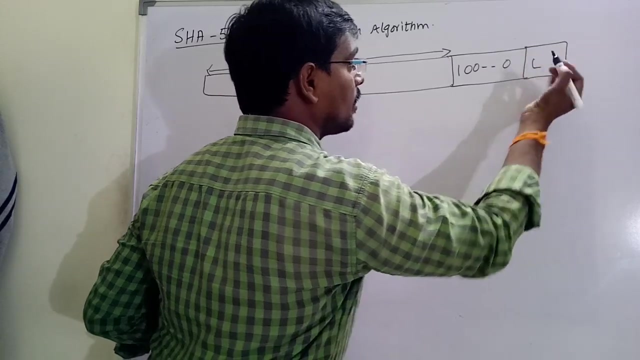 multiple of, for example, number of bits are some l bits. if our message is l bits. if it is not multiple, what we will do. i am doing, padding after padding, i will add 138 bits. after padding, i am adding 128 bits at here. so in this l bits, i am adding 128 bits. 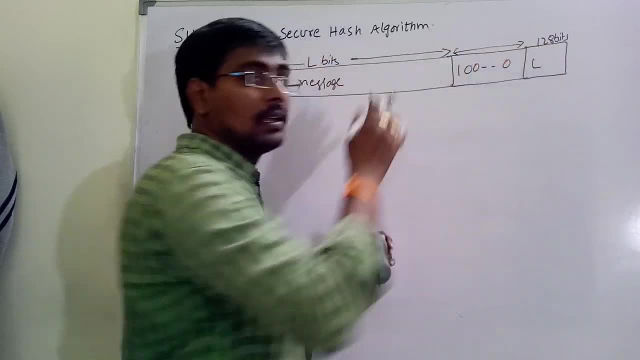 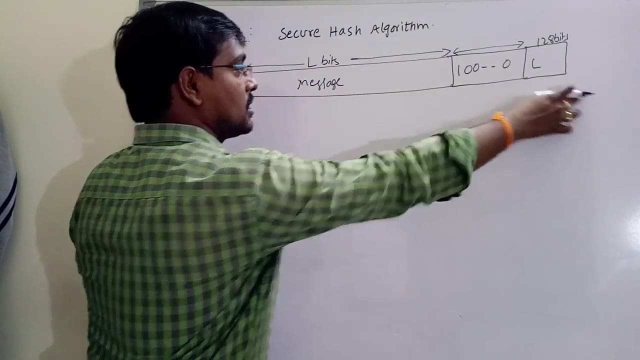 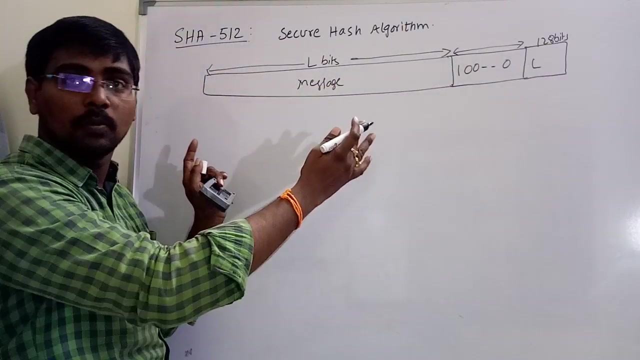 so here i am applying in this position, i am applying padding. now you got it, now total. this is our original message. now, actually, this is the message after performing step one, step two. this is the original message. how many number of blocks? suppose? we don't know number of blocks. 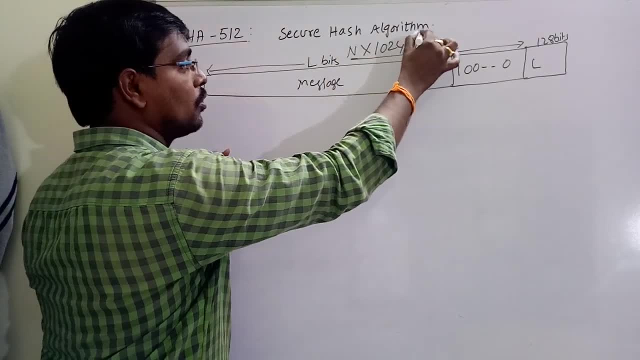 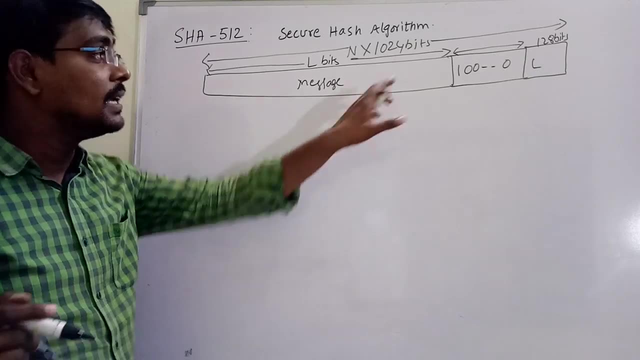 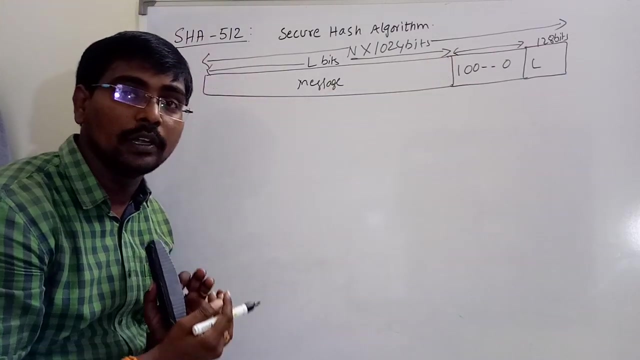 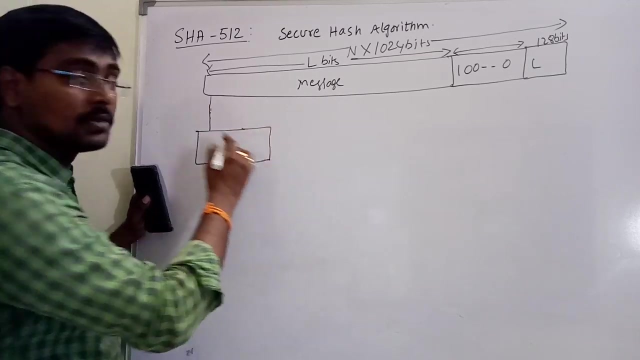 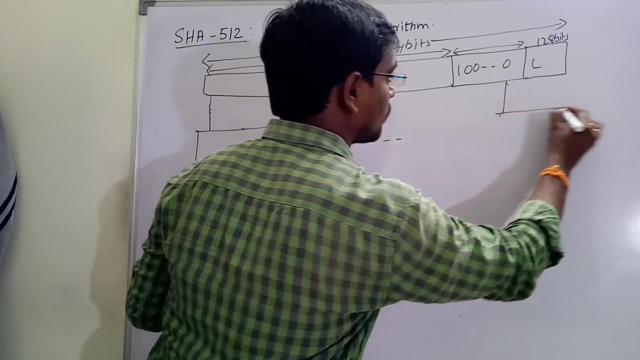 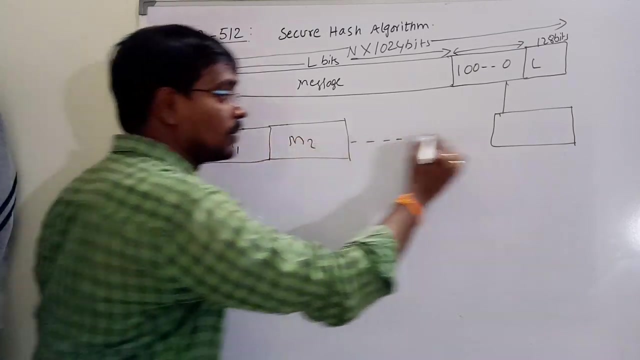 end into 1024 bits: the size of entire message. the size of entire message is multiple of 1024 bits. now what we will do. this entire message is divided into different number of blocks. this message is divided into different number of blocks and so on. for example, blocks m1, m2, m3 and so on. mn size of each block is what is the size of each block? 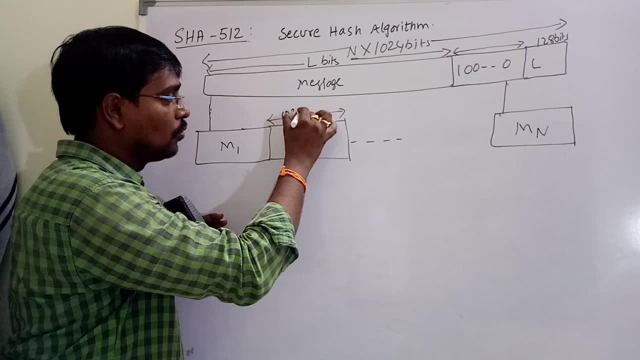 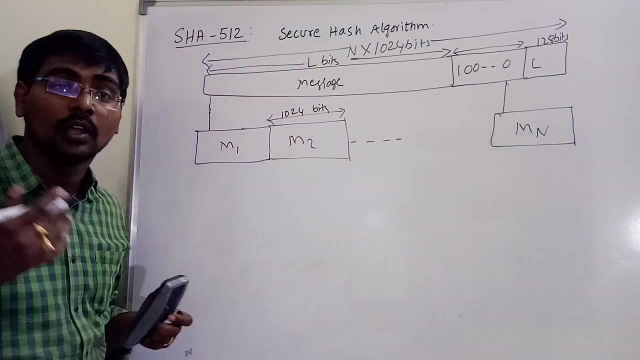 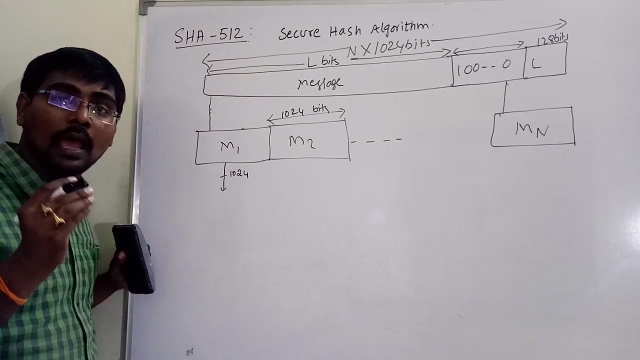 size of each block is 1024 bits. we have n number of blocks, so each block 1024, 1024 and so on 1024. now what we will do on each block, that is, the number of bits, are 1024 on each block we are. 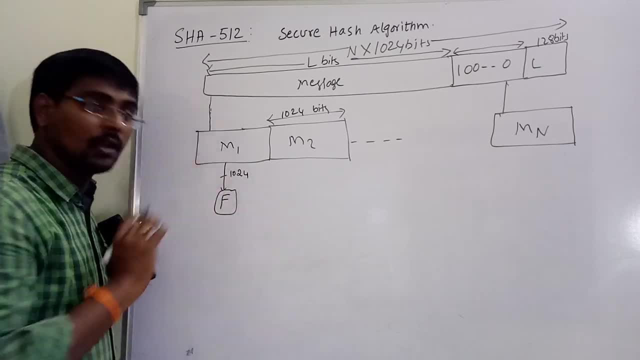 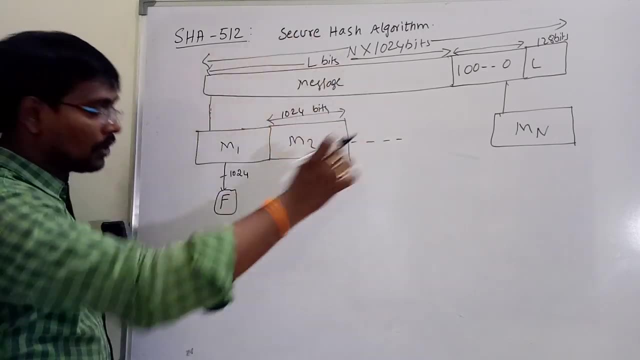 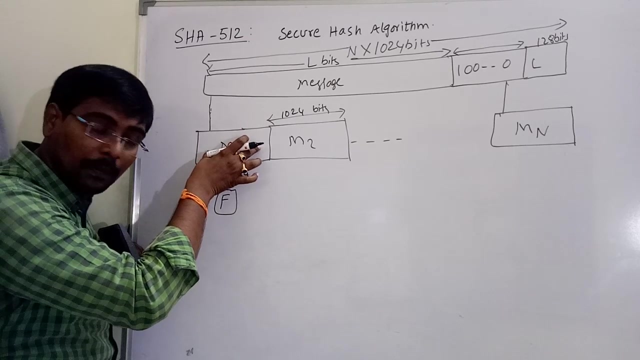 applying a function f. we are applying a function f. what are the inputs? next we will discuss what we will do in that function. this is the overall diagram. what is the input for this function? input for the function is our block, that is our plain test and initial vector: randomly, we are. 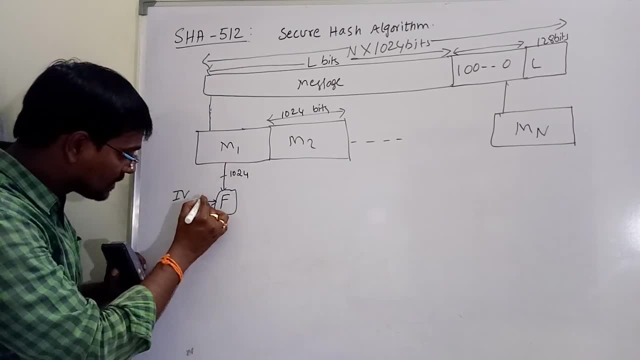 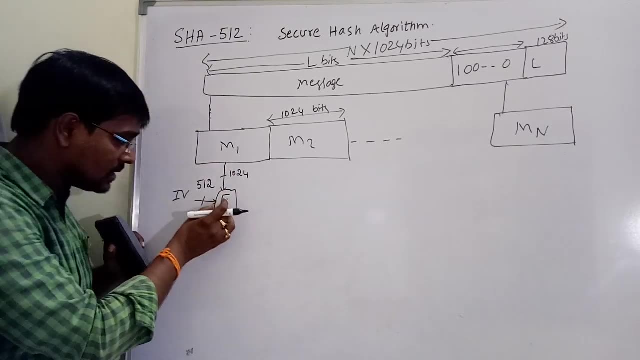 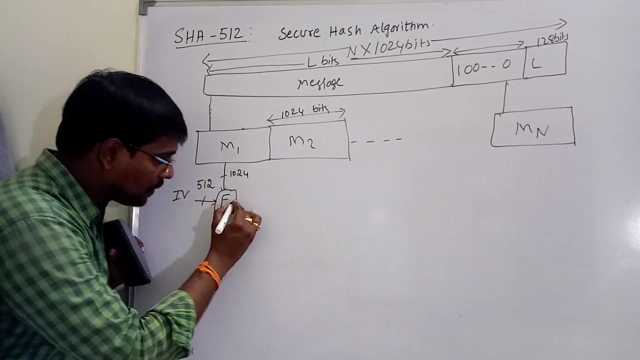 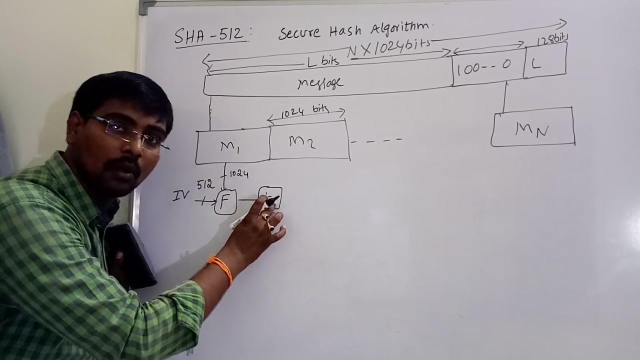 choosing some initial vector and the size of initial vector is 5- 12 bits. the size of initial vector is 5- 12 bits. this is input. this is input after completion of this one. after completion of this one, what we will do, perform. this is not XOR operation. this is addition. modulo 64 addition. 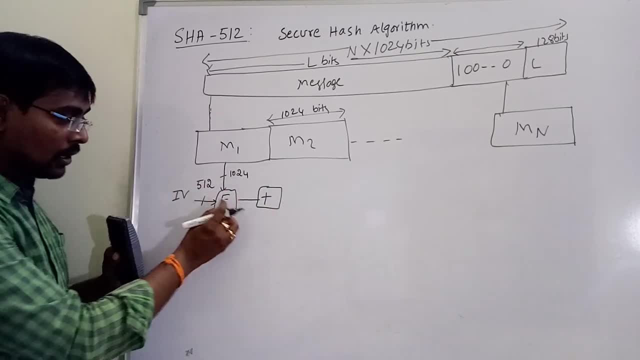 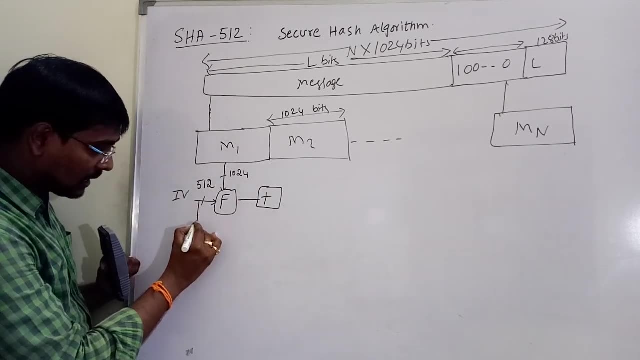 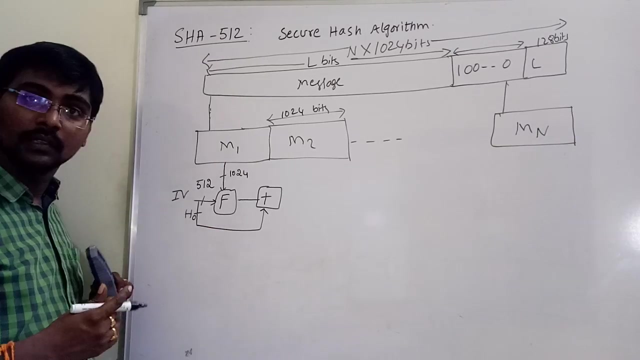 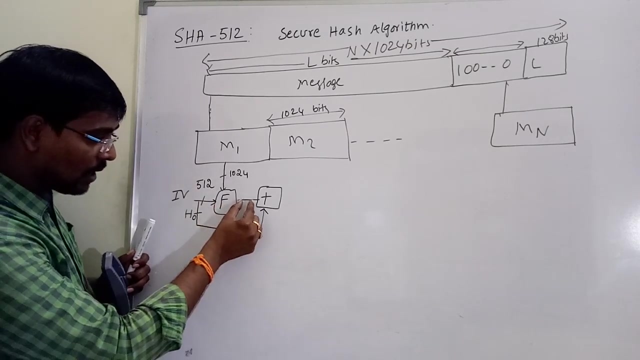 modulo 2 power 64. but to perform operation minimum two operations required. one is output of f, second one is this: one suppose initially this is called some H naught, that is, hash 0 output. hashing is H naught. so after applying function f we are getting some output. this output and the previous H naught we 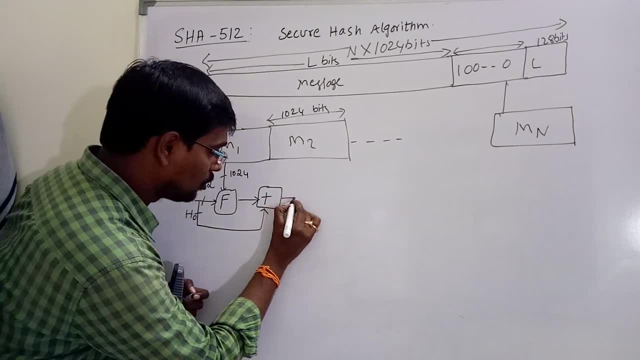 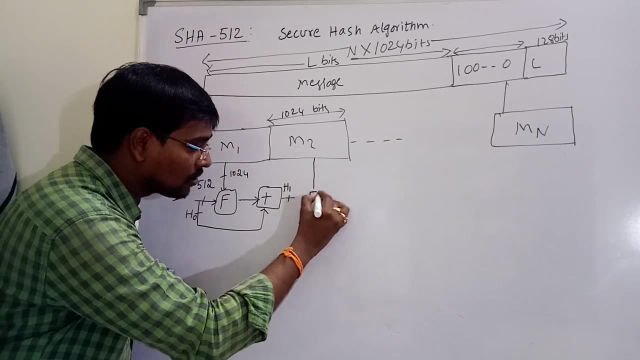 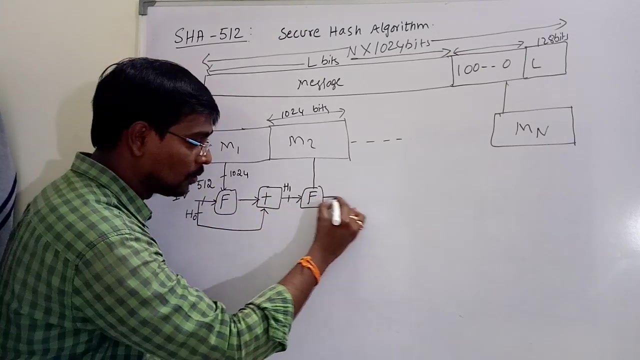 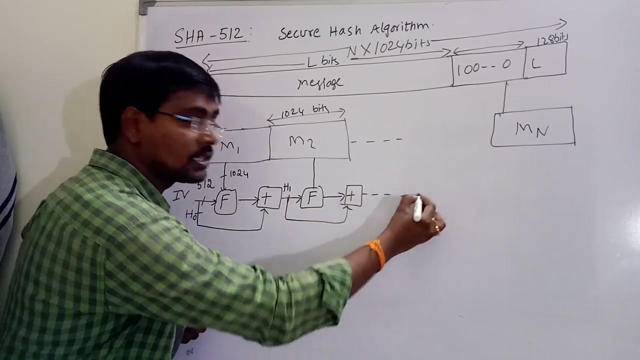 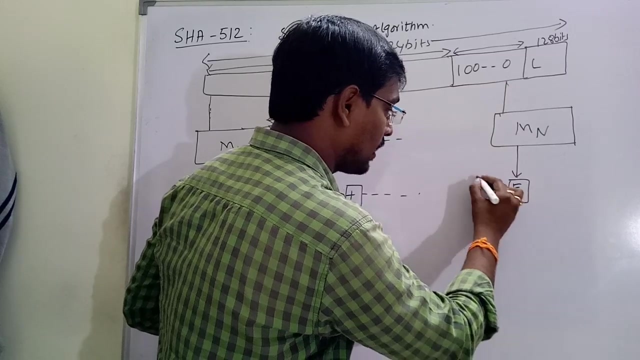 are performing modulation. now it produces, suppose it produces H 1. so the same logic: now the function f and this H 1, all the upper function of, and this H 1, it produces some output. this one end, this one. so the same procedure is repeated. for example, here we are getting cite N minus one. 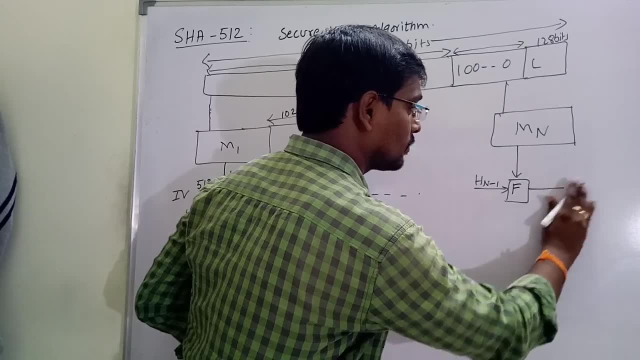 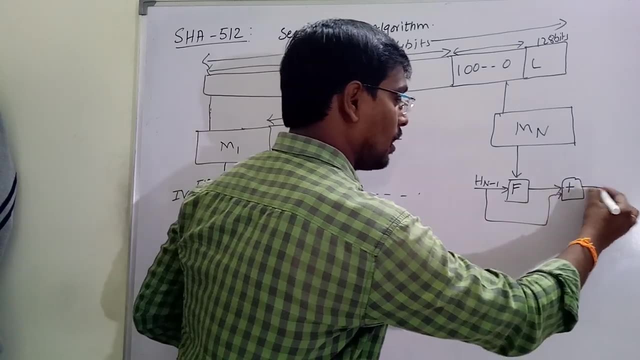 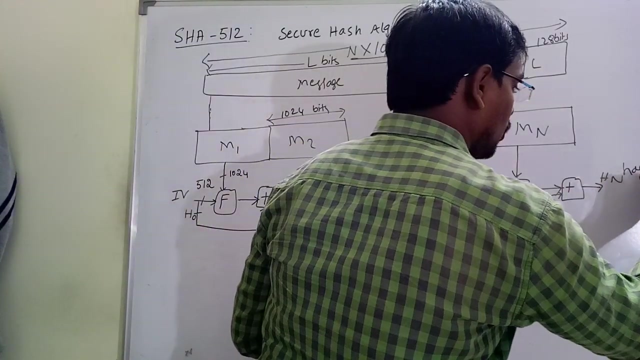 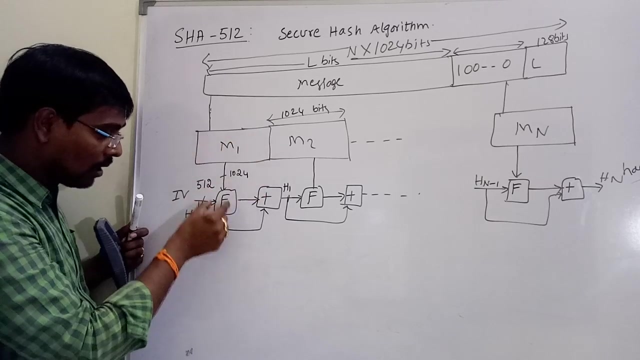 Oh, yeah, yeah, yeah, We are getting some HN. After performing all the operations, we are getting some HN. This is the hash code. This is our required hash code. Observe: The brain test is divided into blocks. On each block, I am performing a function F. 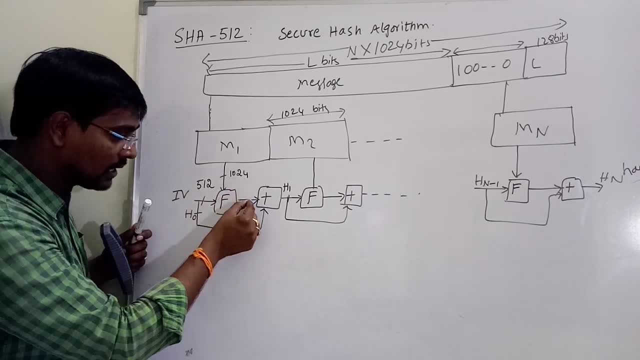 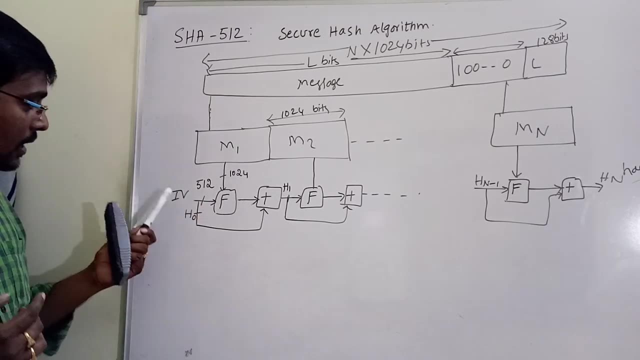 On each block. I am performing a function F. It generates some output And this output, addition model 2464- with initial H0 value, Initial H0 value: Here IV. IV is the initial vector. IV is the initial vector. 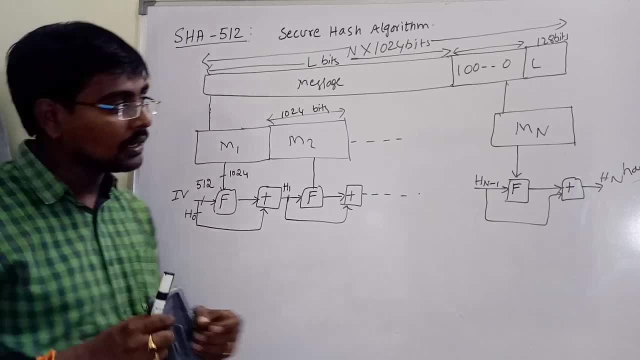 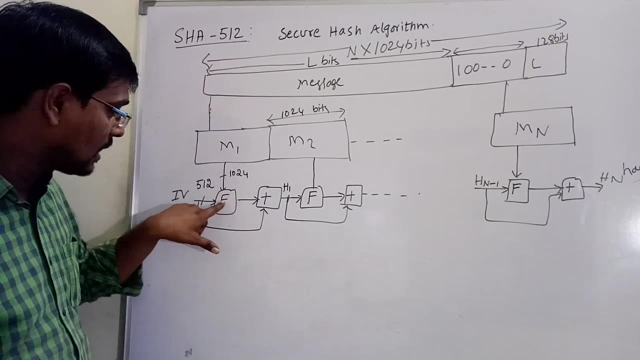 This is the diagram, So observe, We are getting hash code. Now we will move to what we will do on each round. What is our task on each round? That is, on function F. what we will do Now we will move the round function. 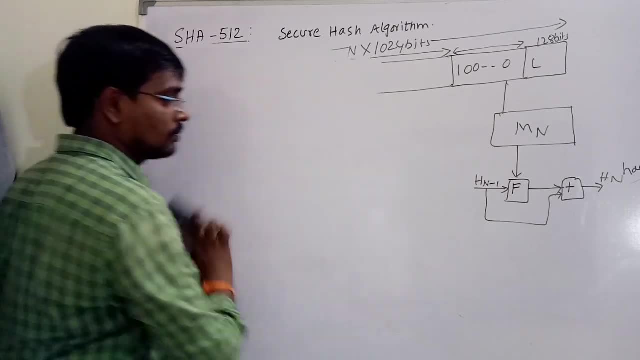 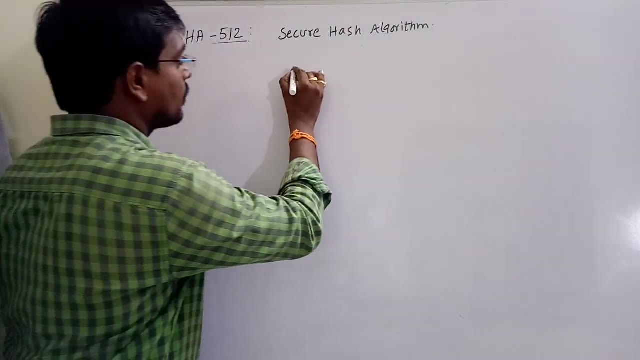 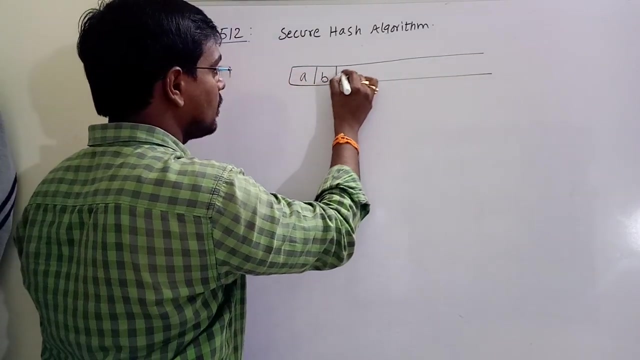 Okay, it is clear What is the round function. Round function is In the round function, that is, in the F, what we will use. I am using the buffers A, B, C, D, F, G, H. 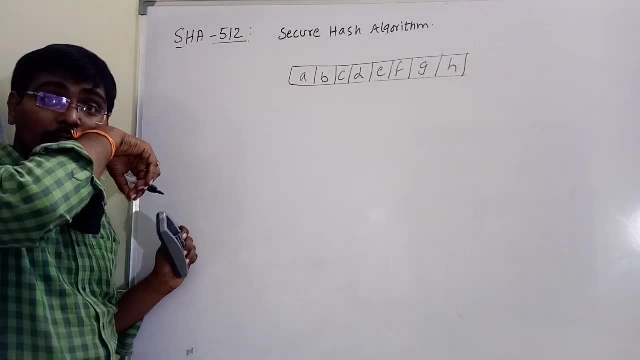 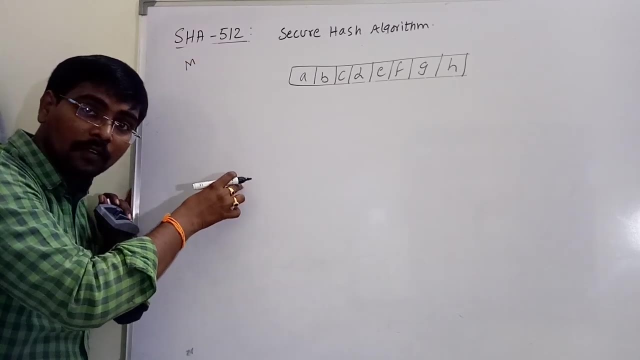 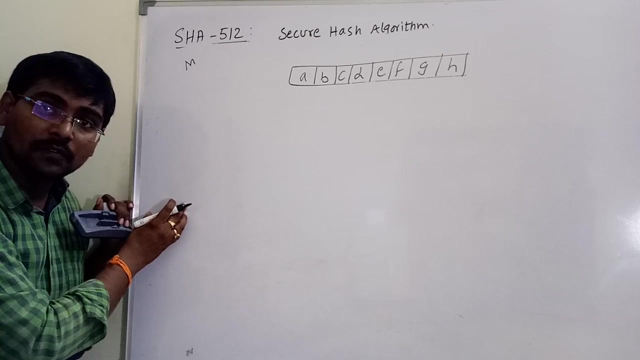 Suppose I am using the buffers A to H, So to provide input. Next, remember the point. Remember, in the function F I am providing one arrow, that is YUM. One input is from YUM, Another one is from initial vector. 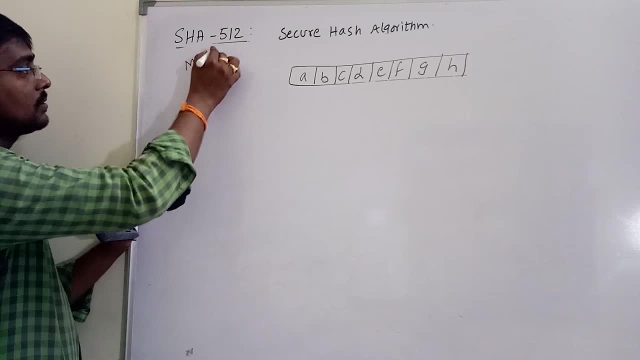 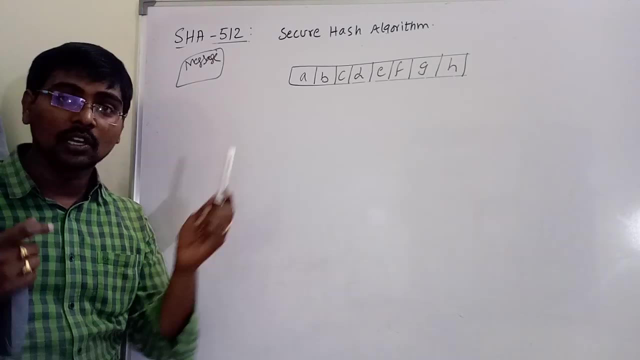 So I am getting message. This is the message From the message in the algorithm we will discuss In each round. in each round, we are generating a word. In each round we are generating a word. Suppose the word name is Q. 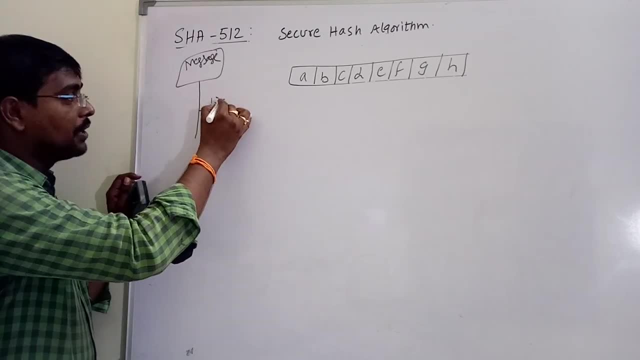 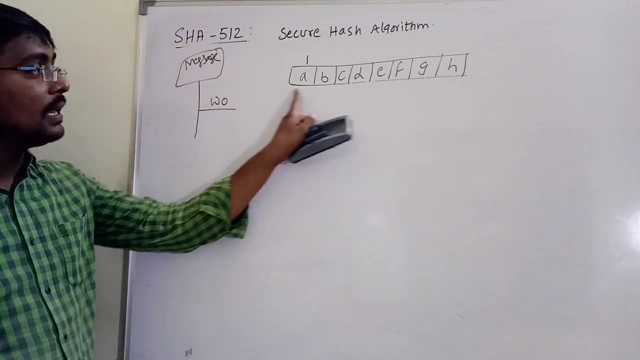 Q word: First round: W G O. First round: W G O. What is the input Here? A, B, C, D, F, G, H, All are called inputs. All are called inputs. 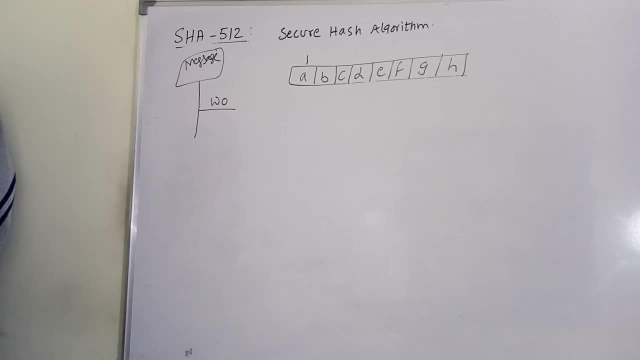 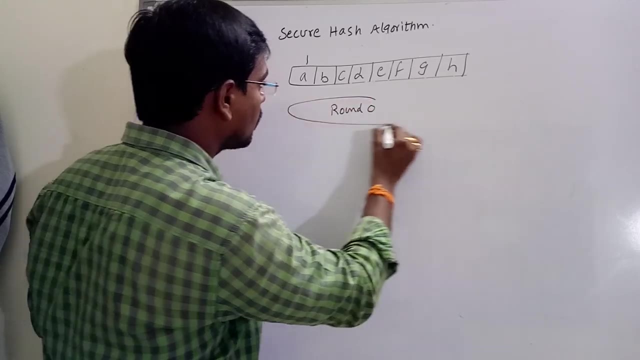 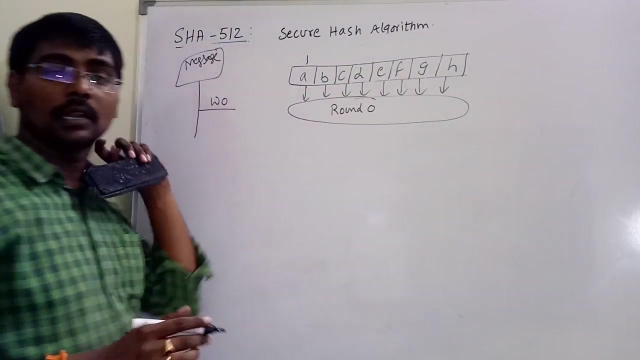 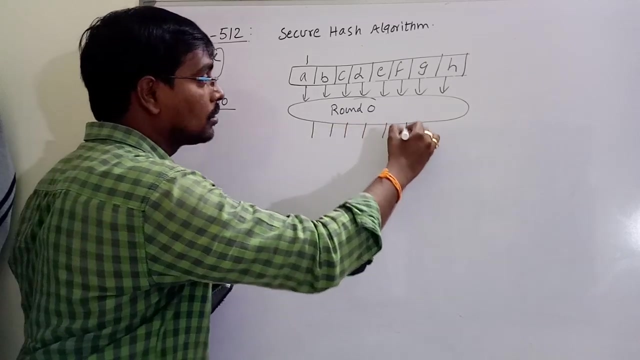 All are called buffers. A to Z are called buffers. Suppose all these buffers are applied for round 0. The buffers are applied for round 0. And after completion of round 0, it produces some output. So for round 0, this is input. 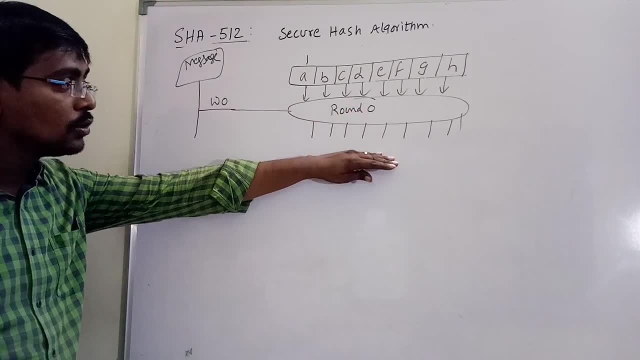 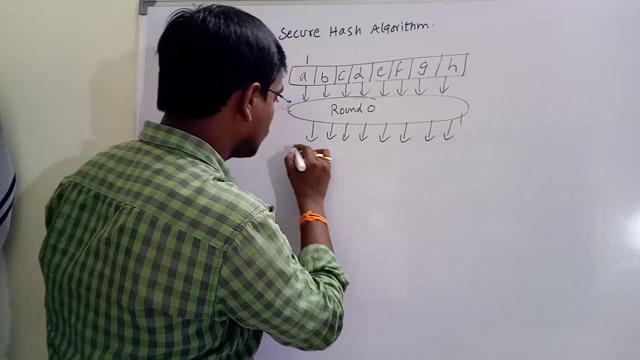 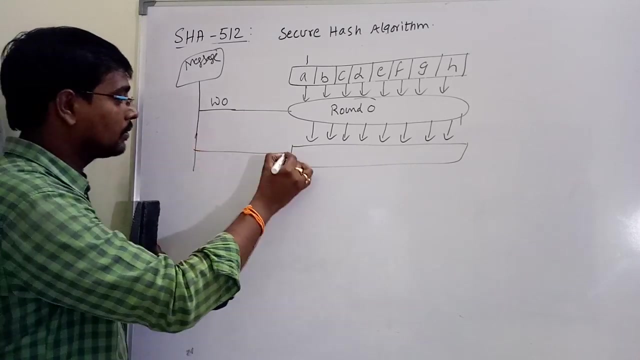 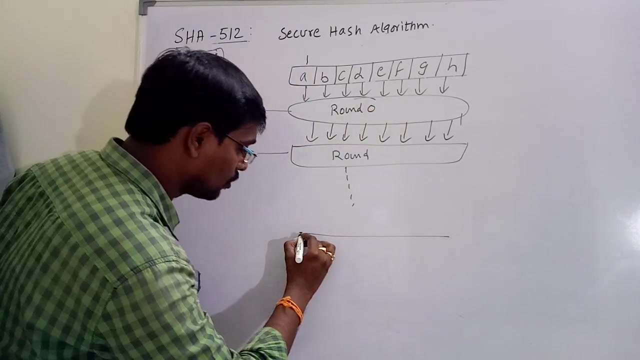 After completion of round 0, it produces some output. This is: This is input to the This output. This output is input to the round 1.. Round 1, and so on. And last one is: We are starting from round 0.. 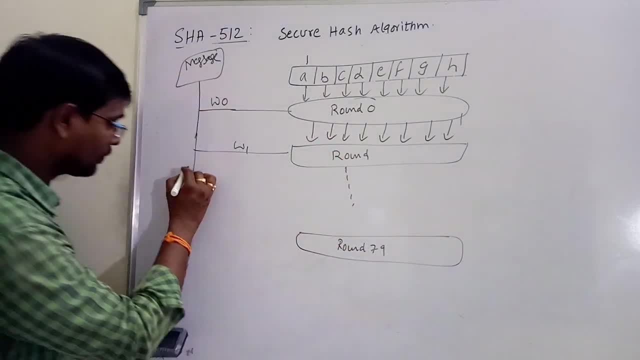 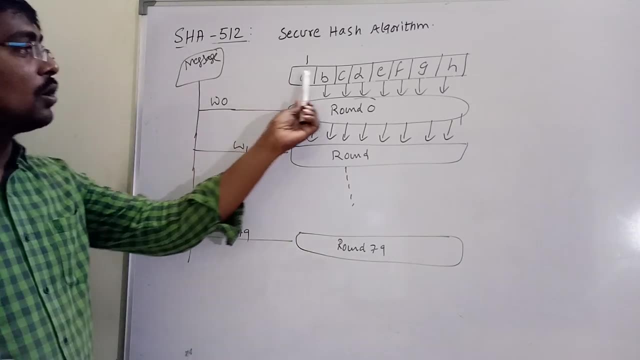 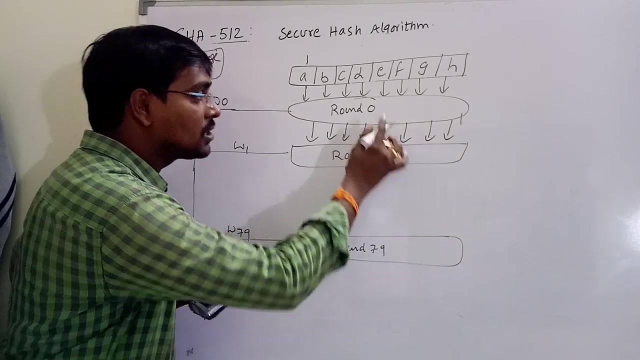 And last one is Round 79. Here diagram is not completed, clearly W79.. So observe: in each round I am using buffers to store the temporary, to store the intermediate results. After completion of one round, we are moving to next round. 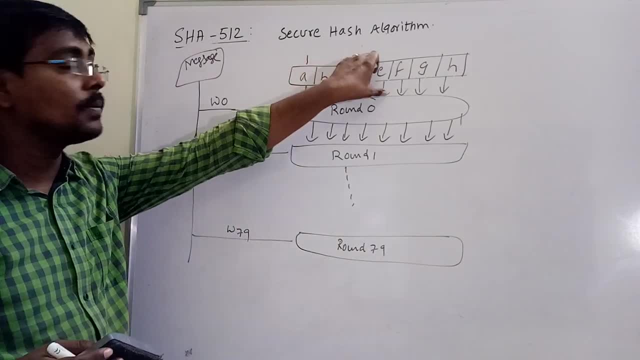 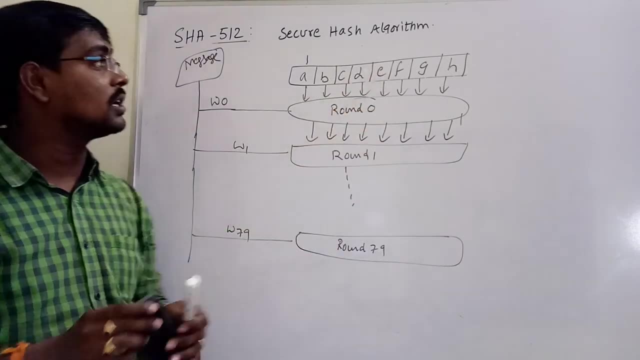 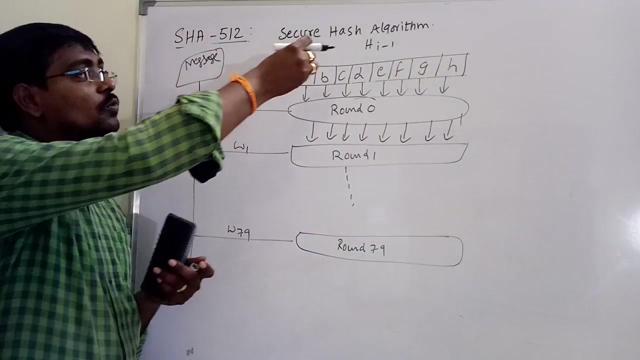 And what is the input to the buffer? In the previous diagram we are using H0.. The input for round 1 is H0.. So I am providing, suppose, HI-1.. If you are using the first block, H1-1, H0.. H2-1, H1 for the next round. 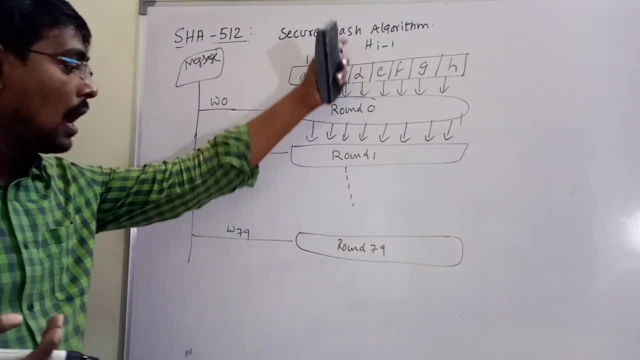 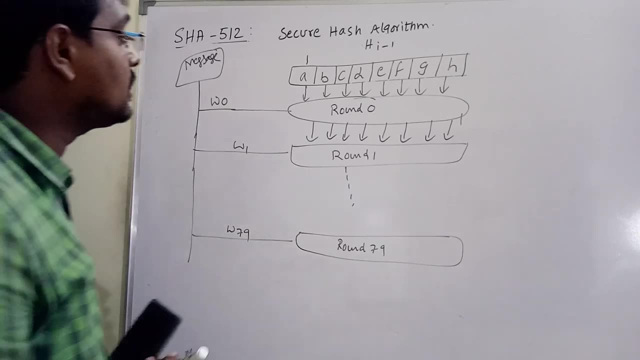 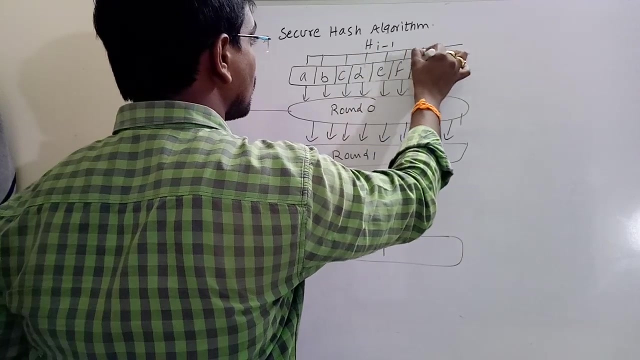 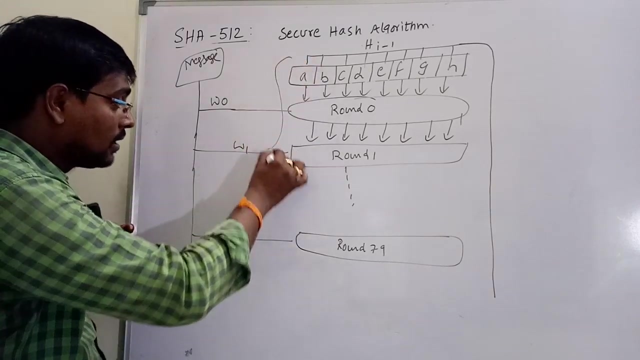 So I am using HI-1 after completion of all rounds. After completion of all rounds, What it gets, It gets HI. So suppose this one, What we will do After this entire thing is F. Remember, this entire thing is F. 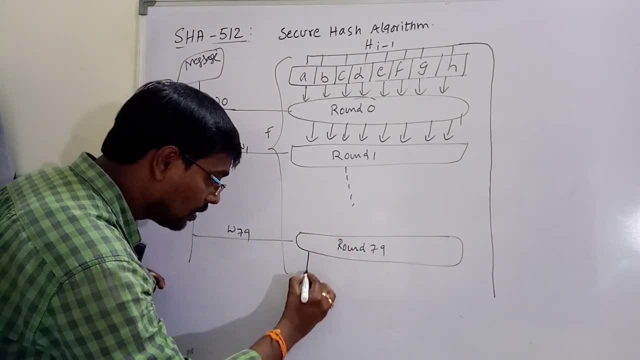 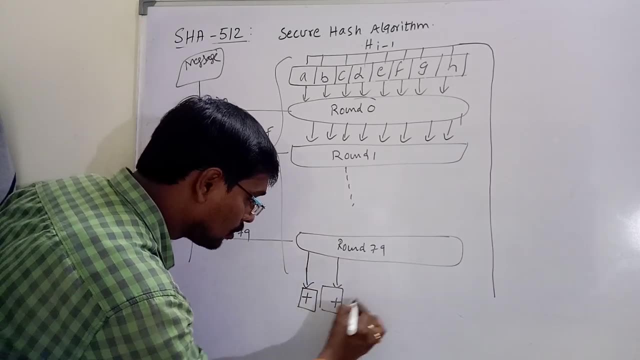 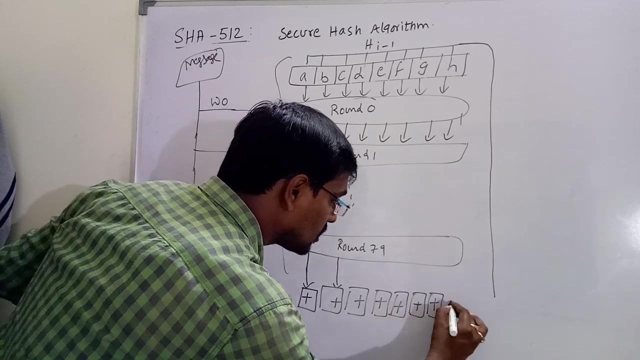 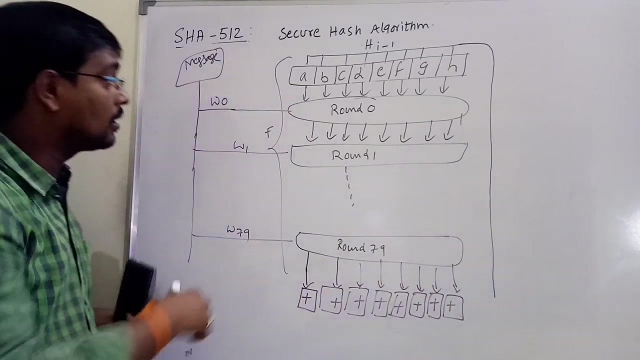 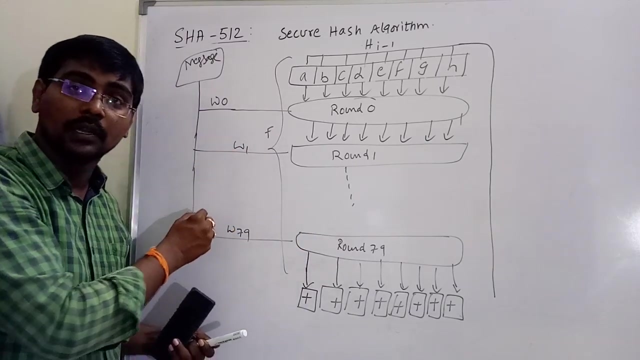 After completion of round 70,. we are applying this operation. I think you got it: 1,, 2,, 3, 4,, 5,, 6,, 7, 8.. So I think you got it. All these round 0 to round 9 are F. After completion of F. after completion of F, we have two inputs. What are the two inputs? 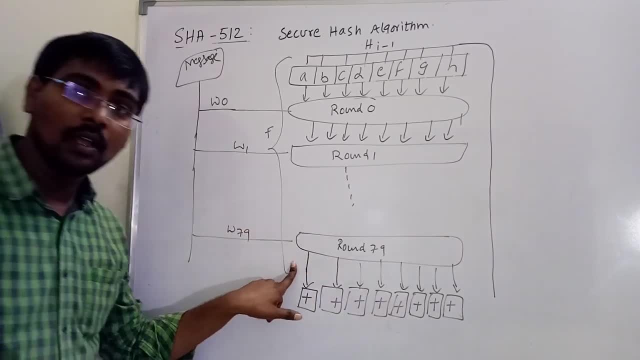 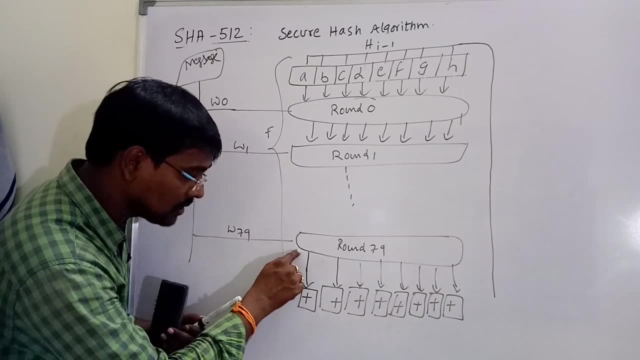 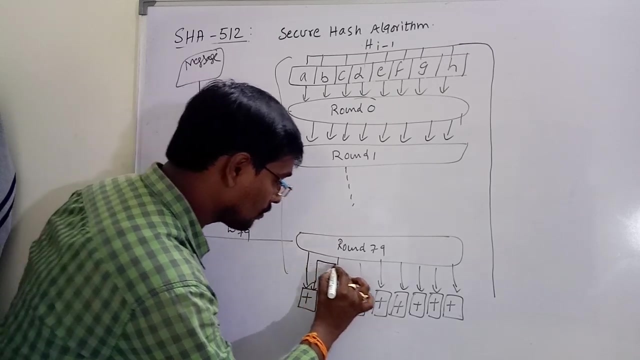 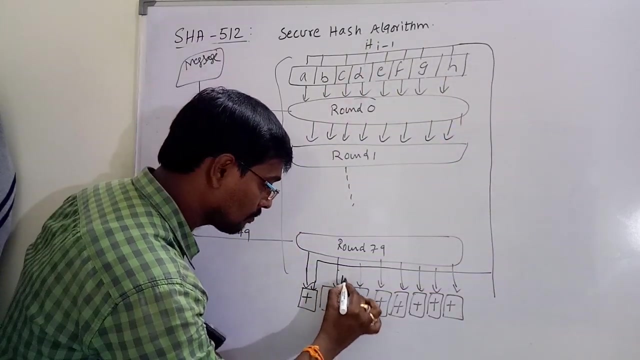 One is output of F. One is output of F. Second one is H0.. So this is H0.. So for F, input is output of F, is this one, and so this is H0.. This is H0.. I think you got the point. 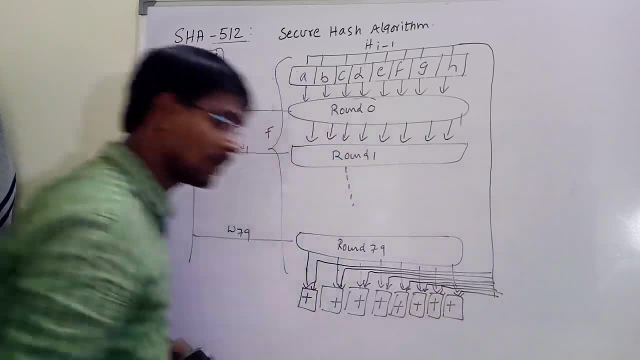 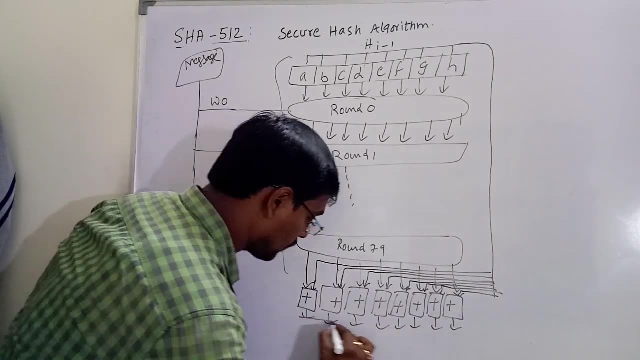 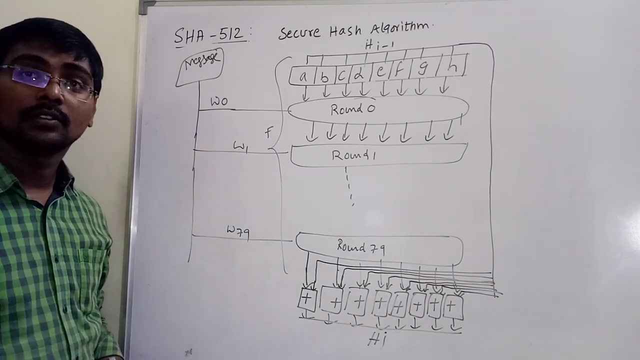 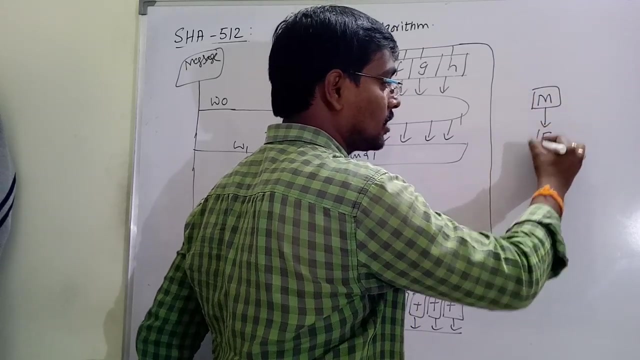 You got it. After completion of all this, what we will get After completion, we will get H1.. That is HI-1, HI, HI. So in the previous one, what we will do, M For this M, I am getting the function F. 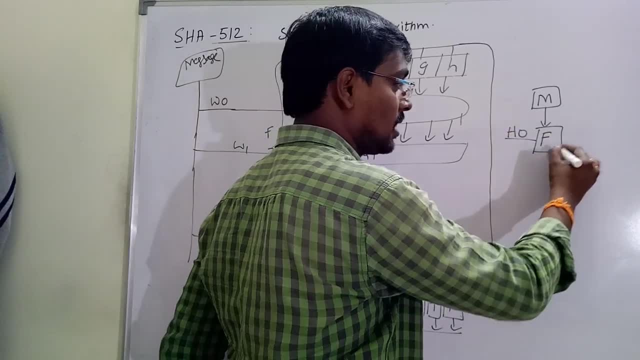 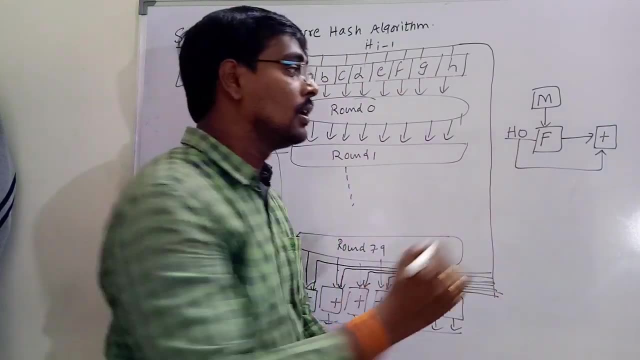 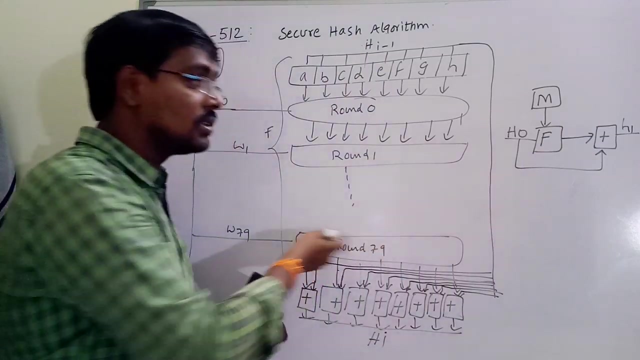 Function F. I am providing H0 as the input. It provides H0.. It provides some output. This is we are doing. It will produces some H1.. After applying, it produces H1.. So here, this is our case. 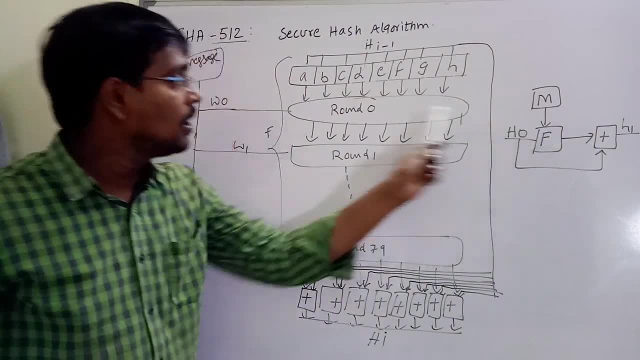 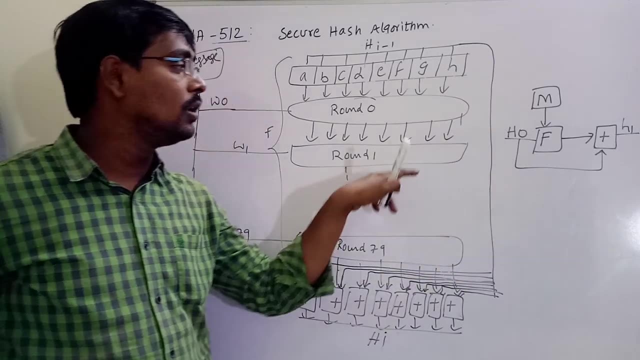 Here this is the case And each F we are performing 80 rounds. For example, we have 4 blocks in our algorithm. We have 4 into 80.. 320 rounds are performed. So F, this is round 2.. 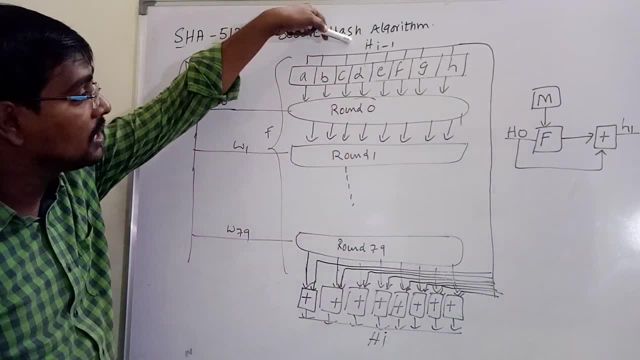 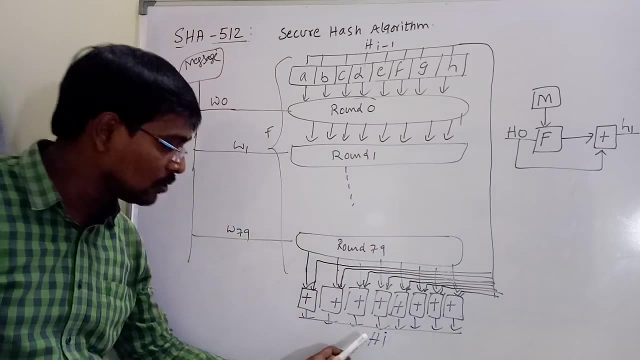 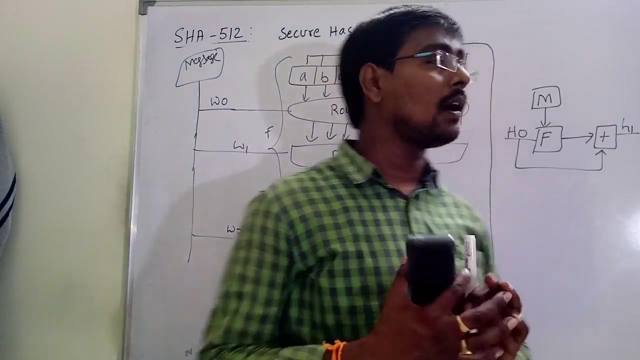 Round 17 and F. H0 is the initial hash code and XR operations. the input is output of F plus H0, it produces H1.. This HI is moved to second block. That is moved to next block until completion of all the messages. 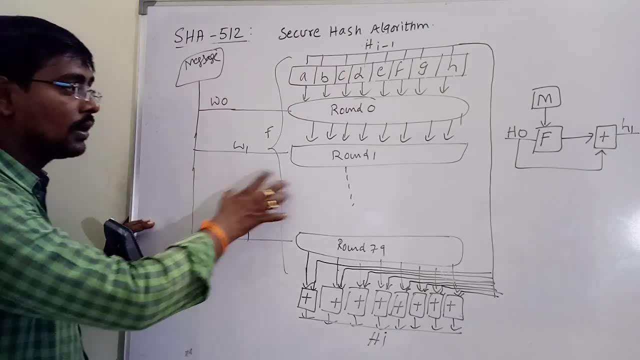 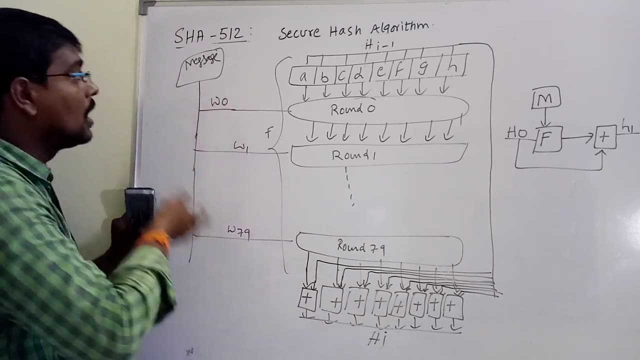 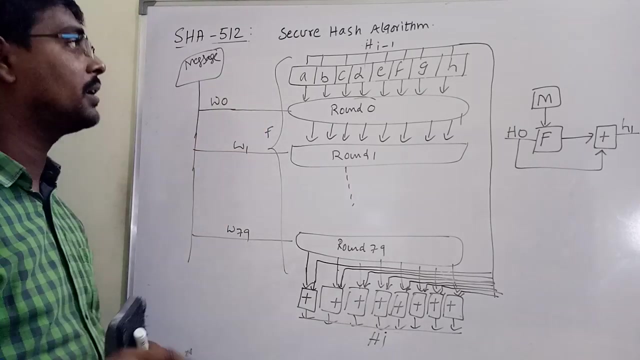 Okay, This is the secure hash algorithm block diagram and then each round operation. Next we will move to: in each stage we are developing watts, How we are generating the watts. Watts are generated from playing test. Now we will move how watts are generated. 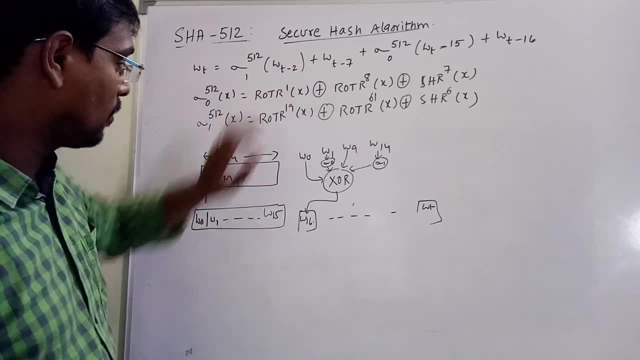 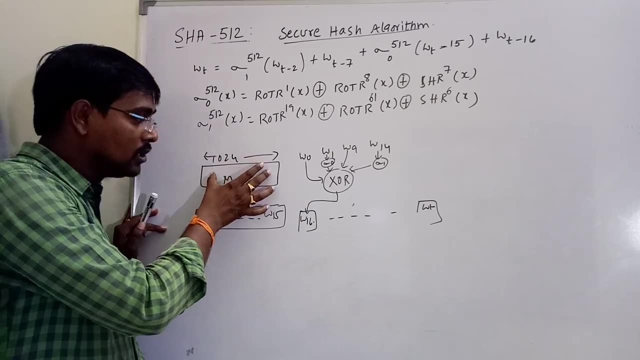 This is the way to generate the watts. This is the formula. For example, suppose we consider block M1.. Number of bits is 1024 bits From 1024 bits, size of each watt is 64. So we are generating 60 watts. 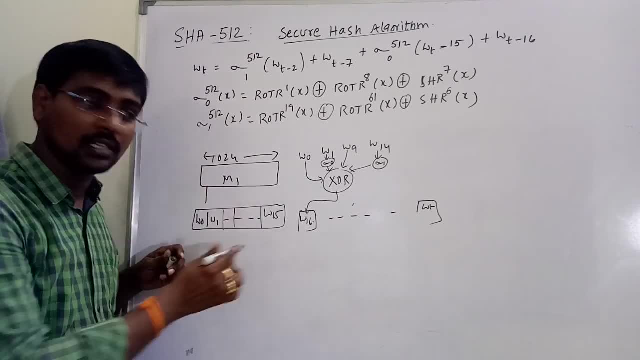 Watt 0,, watt 1, and so on, watt 16. So 16 into 64, 1024 bits, So 1st to 15.. That is sorry, 1st to 16, there is no problem. 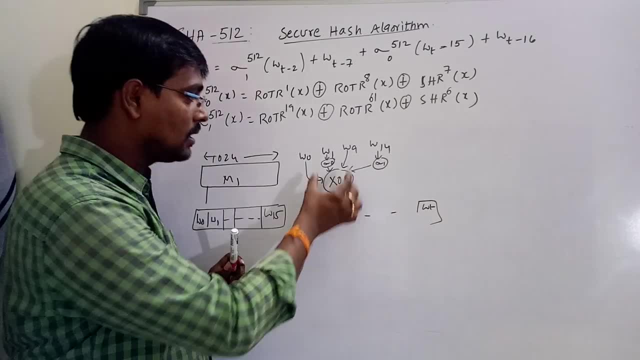 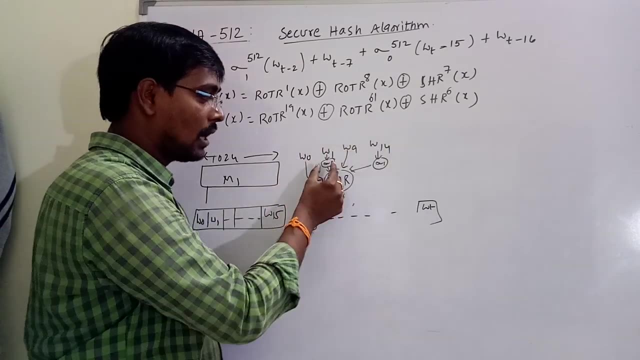 To generate the next 16s. the formula is: consider these watts from the first 16.. W0, W1, W9, W14.. Apply sigma 0, sigma 1 on W1, W14.. Perform XR operations. we are getting W16. 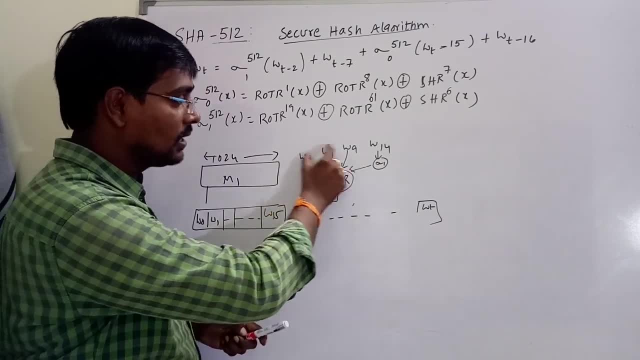 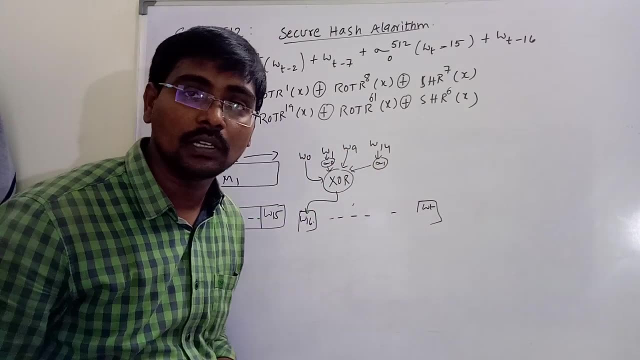 In a similar fashion, we are taking next two bits, A similar next two bits to get W17.. Until our required number of watts is reached. This is the formula. Suppose how to get Wt. Suppose to get W16.. 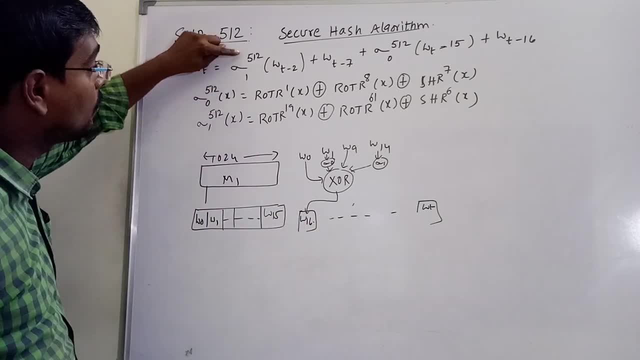 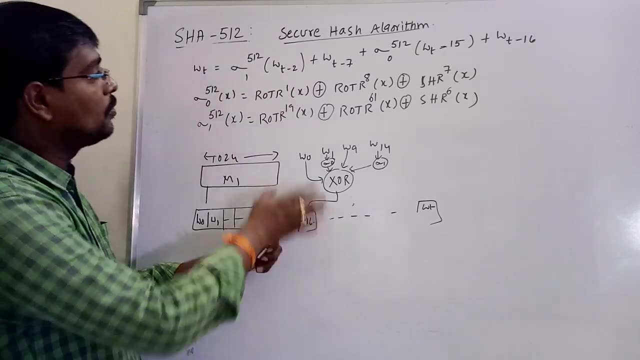 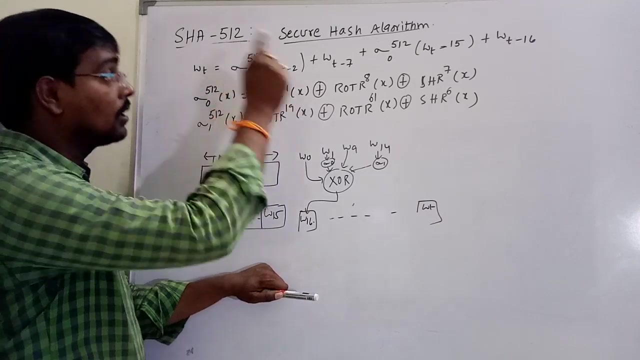 What is the formula? Sigma 1, 512 of Wt-2.. For example, to get 16, to get W16, we are using W14.. So observe, we are using W14 on sigma 1 function And Wt-15,, that is, 16-1,, W1 on sigma 1 function. 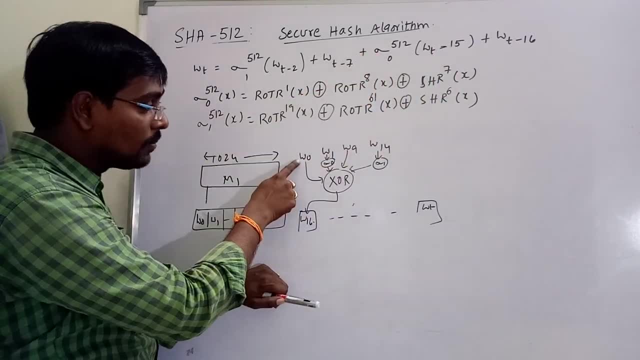 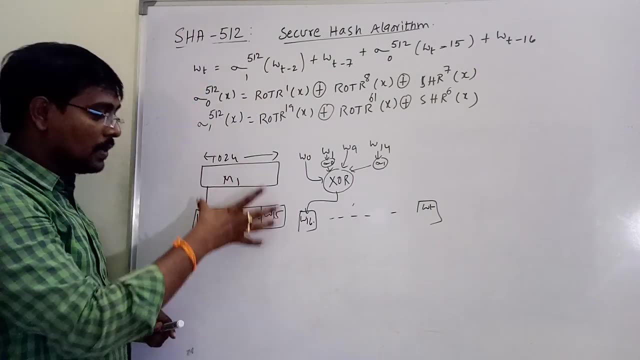 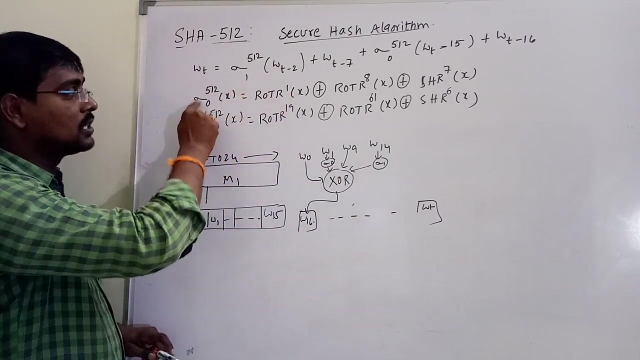 Along with I am using W0 and W14.. That is Wt-7, Wt-16.. That is based on these 16 watts. we are generating new watts. So here, what is sigma 1-2-5-volt? sigma 0-2-5-volt. 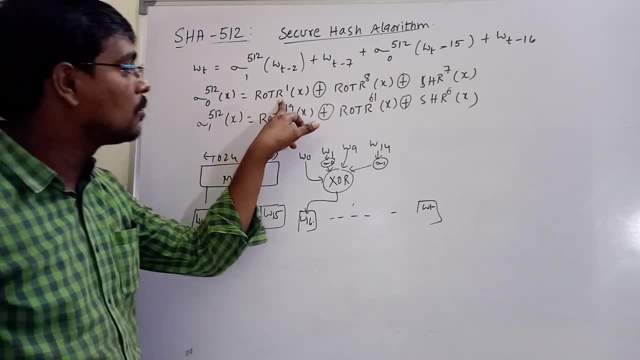 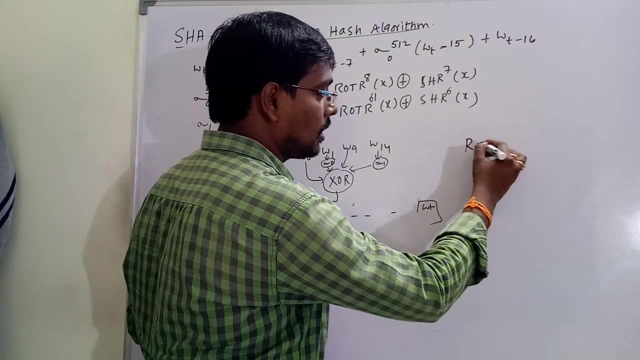 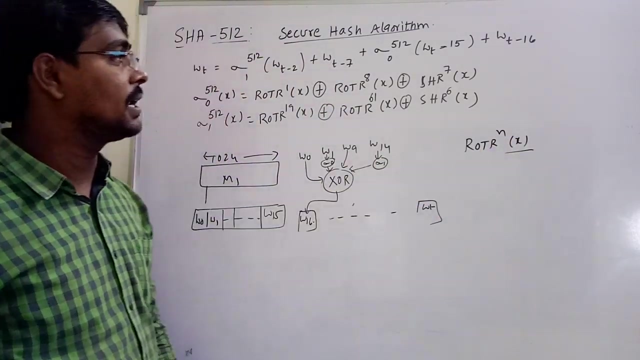 This is the formula. Rotation ROTR means shift right or shift rotate ROTR, for example ROTR N X. Rotate X by N number of bits, Rotate X by N number of bits. So after performing all these operations, we are generating total 80 watts on each round. 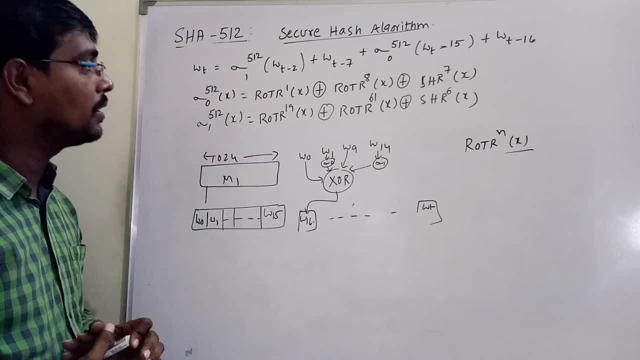 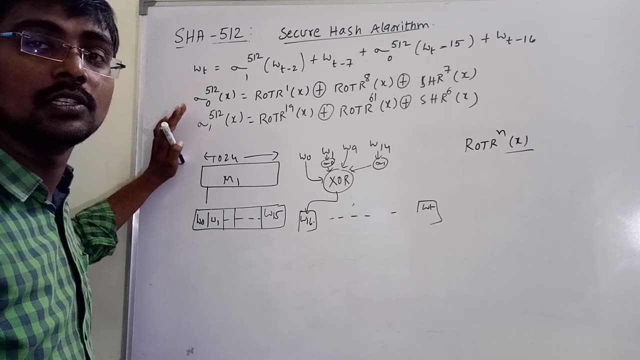 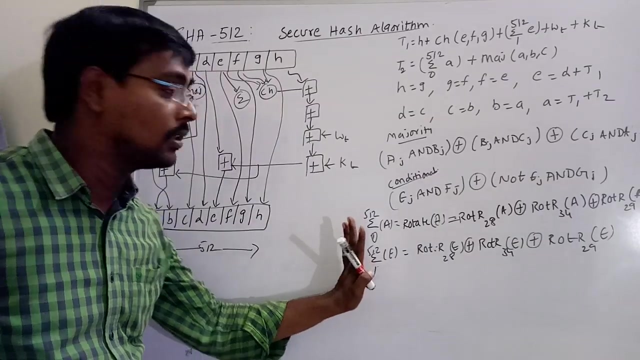 We are generating a total of 80 watts on each round. After completion of this one, how the buffers are changed, How the buffers are changed. We will discuss how buffers are changed in this one On this awareness. finally, what happens on each round. 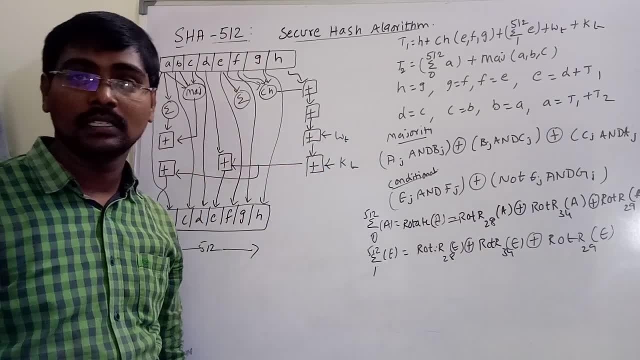 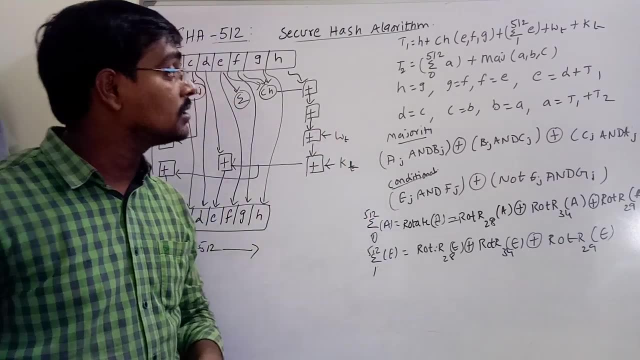 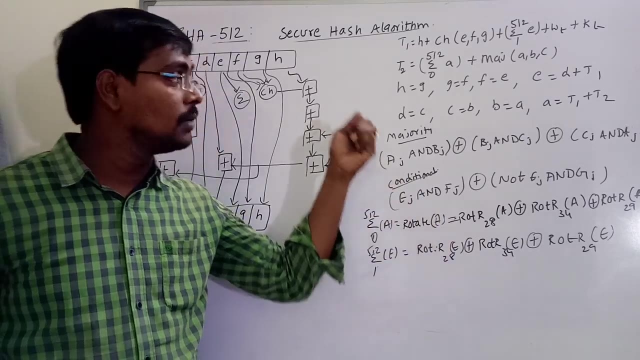 Each round we are generating 80 watts. At the same time, each round we are generating 80 constants. Here, K means a constant, KT means constants. This is the procedure That is, between these buffers, one buffer to another buffer. we are providing input to the first buffer. 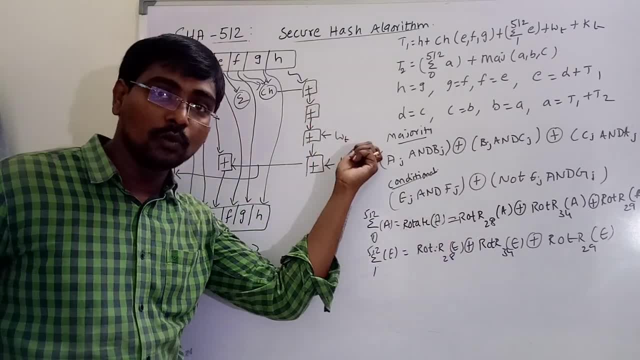 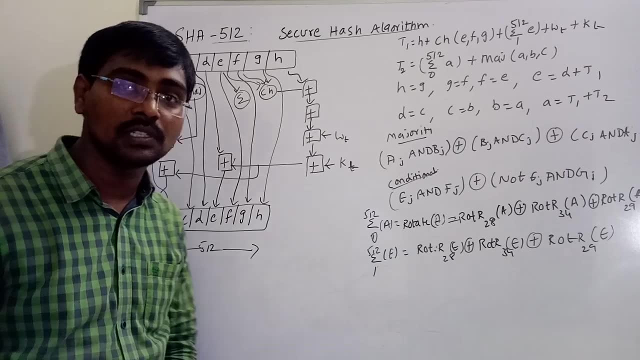 From first buffer output is moved to second and second to third. What happens in between? For these 17 H, 0 to 79, that is 80 rounds. So A to H, these are the 5-volumets. 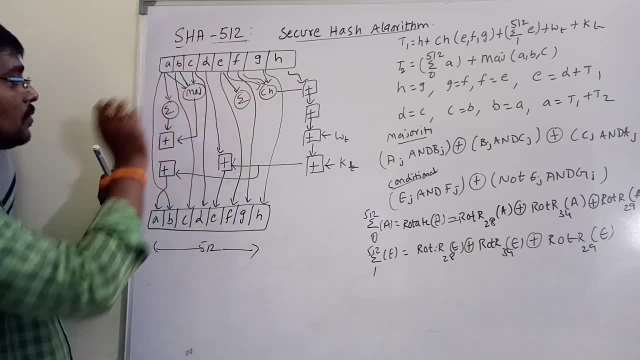 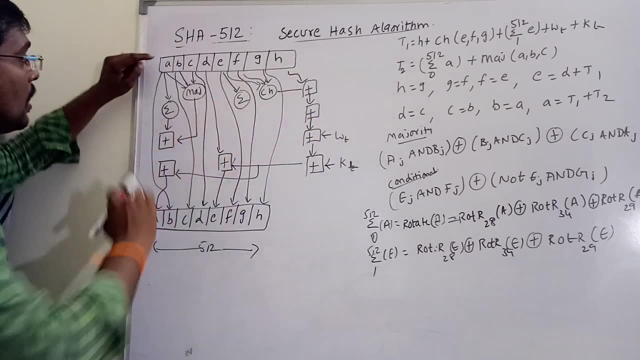 These are the 5-volumets. On these 5-volumets we are generating finally 5-volumets In between these two. this happens. So first buffer A: whatever the value present in buffer A, that is directly transferred to buffer B. 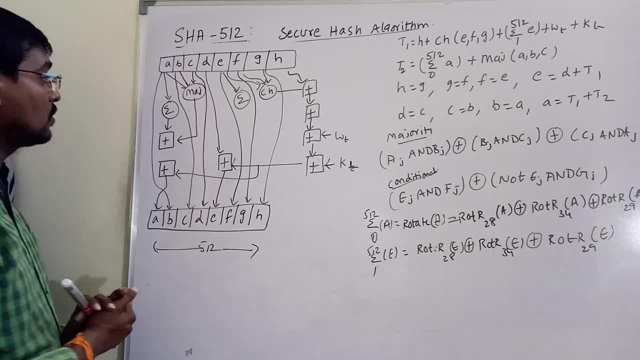 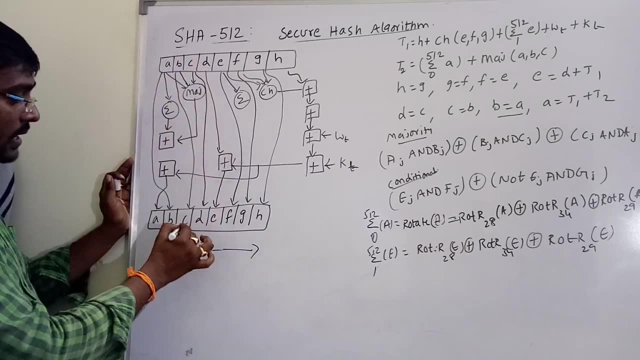 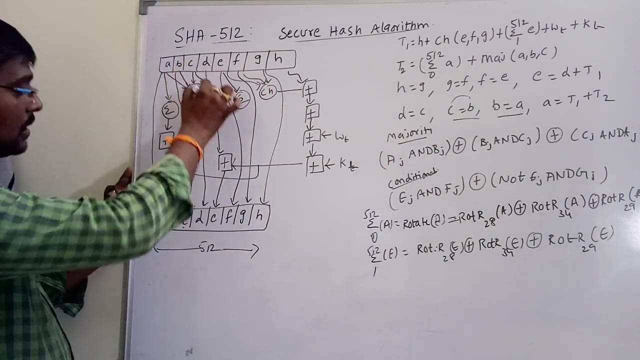 The buffer A value is transferred to buffer B. So this one And buffer B value is transferred to buffer C. So B value is transferred to buffer C And buffer C value is transferred to buffer D. So each step A value is transferred to B. 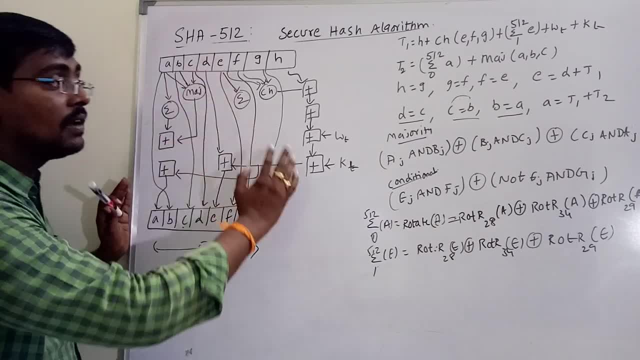 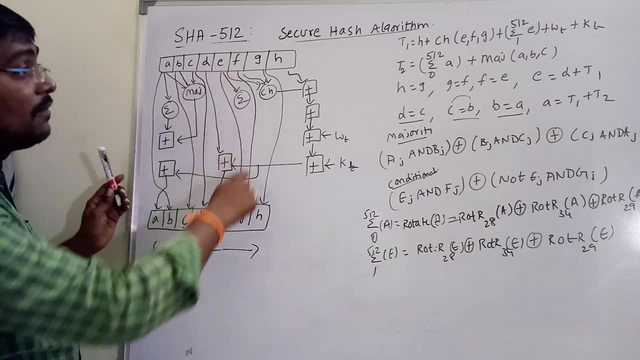 B value is transferred to C. C value is transferred to D. So shift bits, Shift bits And at the same time E value. E value is transferred to D. E value is transferred to directly, not F, E value. 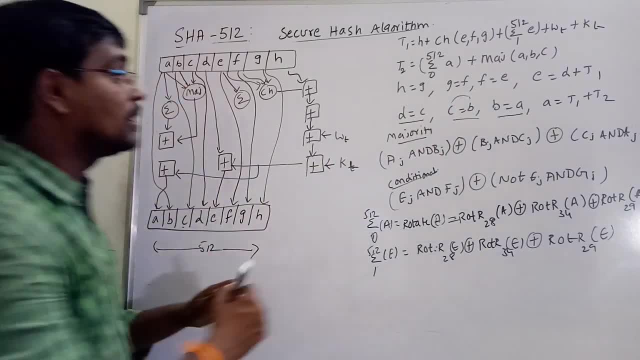 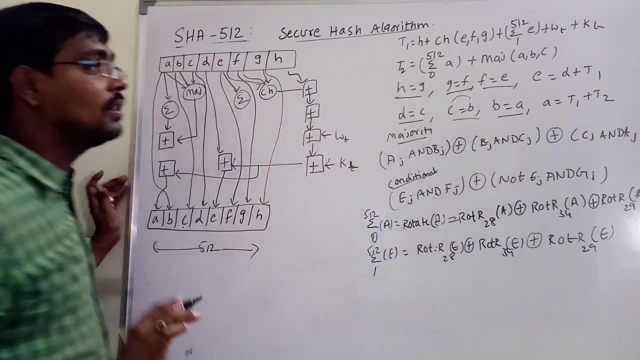 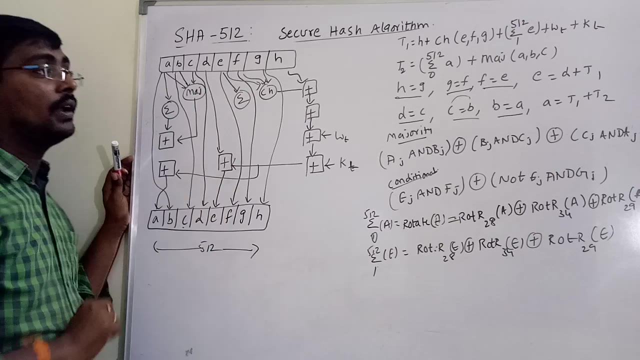 Suppose: see this one: E value is directly transferred to F, F value is transferred to G, G value is transferred to H. All these are okay. What is this one Here? what happens to E value And what happens to A value? 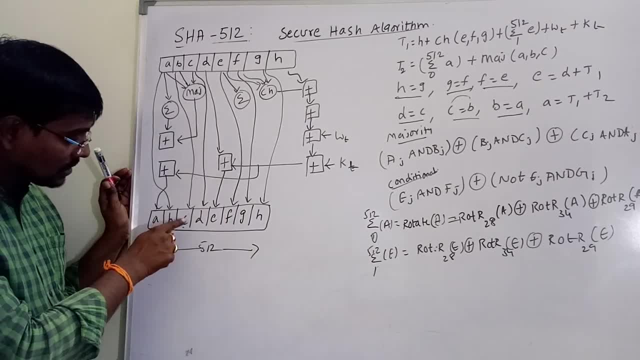 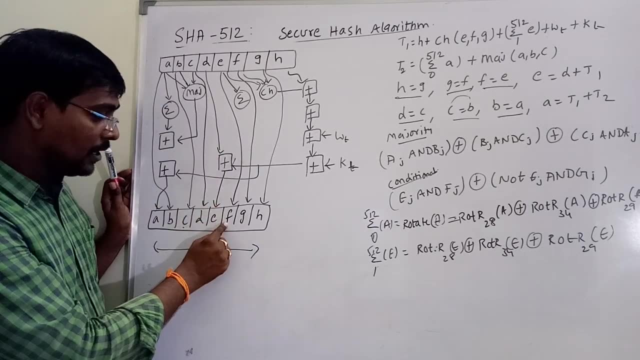 Observe: A value is copied to B, B is copied to C, B is copied to D, C is copied to D. So further E. E is copied to F, F is copied to G, G is copied to H. 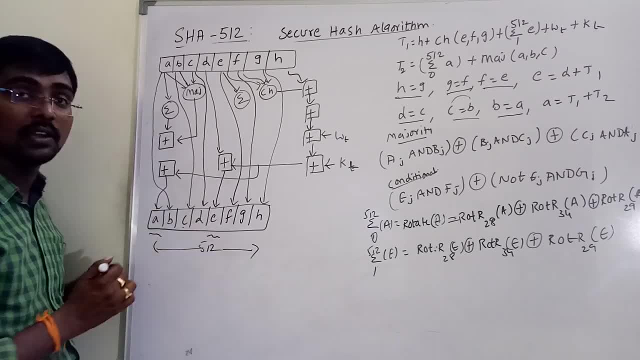 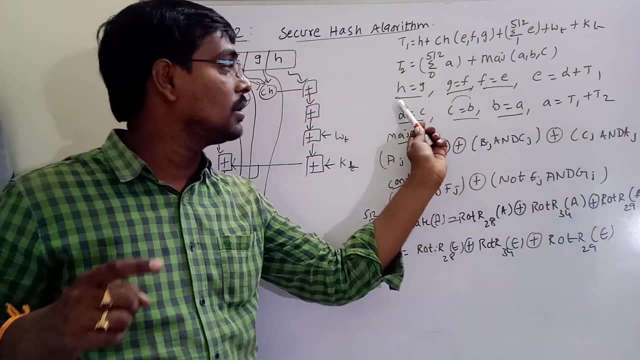 But what about this A value and this E value? First, we are performing this operation. We are following the same sequence. Remember, we are following the same sequence. E is equal to D plus T1.. So this is the first operation. 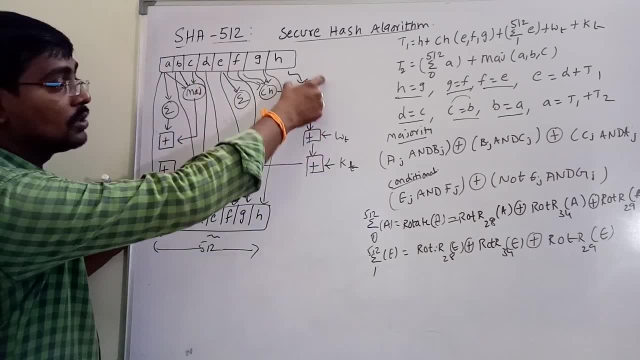 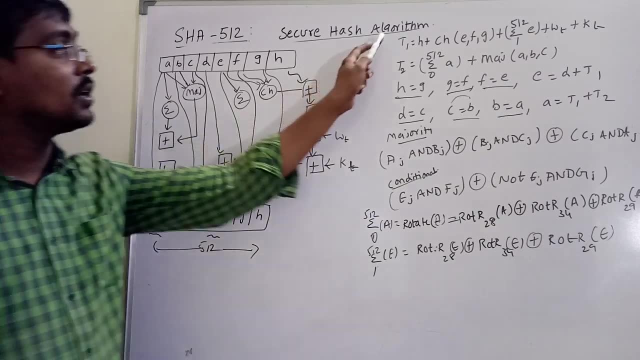 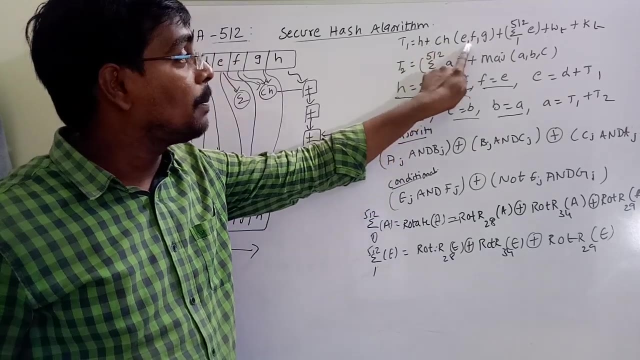 D plus T1.. So these are the words. Suppose we are using kth round, Tk. fifth round, T5.. So what is the formula for T1 and T2? This is the formula H plus. This is a conditional function of buffers E, F, G. 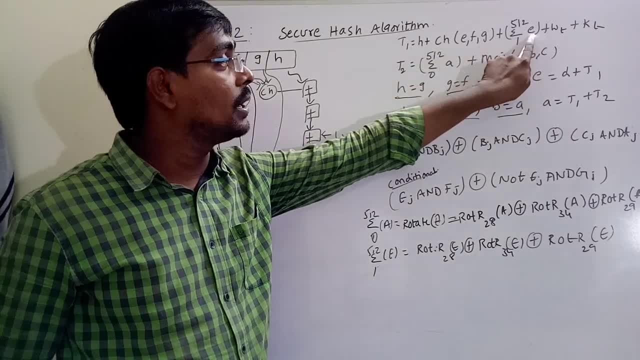 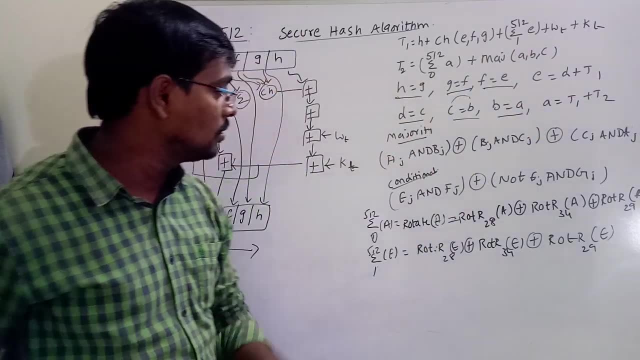 H plus E, F, G For and sigma for the buffer E, Wt plus Kt. Similarly, here we are using some majority function. So these are the formulas Majority function. Here the majority function is applicable for buffer A, B, C. 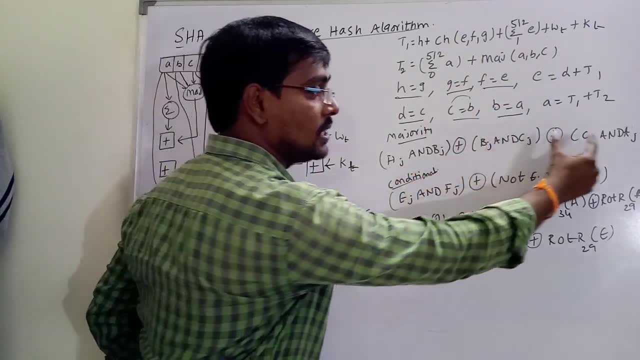 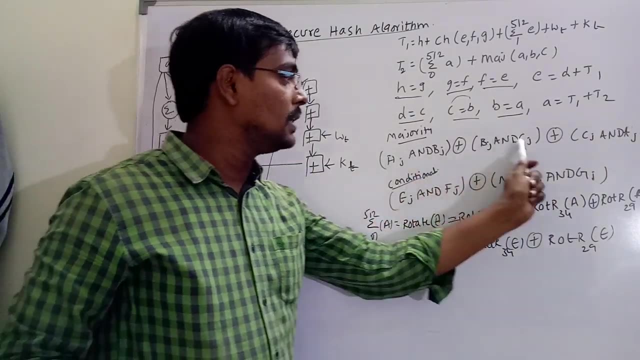 So A and B, B and C, C and J, C and A Between A, B Perform. This is the logical end operation: A, B, B, C, C, A. This is the majority function, Similarly conditional function. 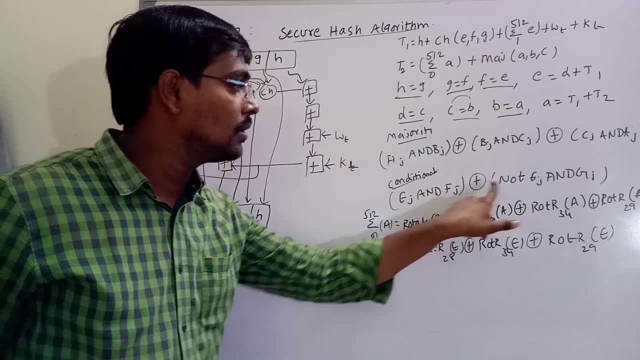 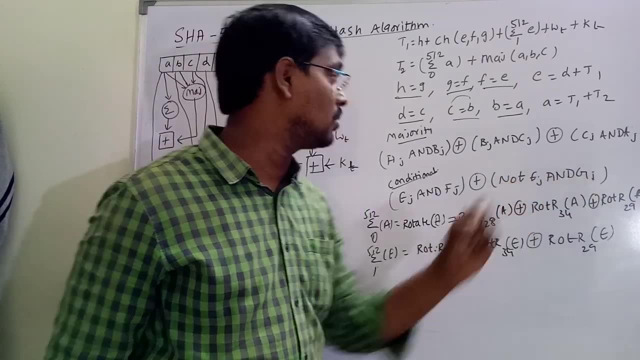 E, F, G, E and F, Not E and J. This is the conditional function, That is, if E is true, not E means false, False and true. And what are the sigma functions? Simply, these sigma functions are rotate functions. 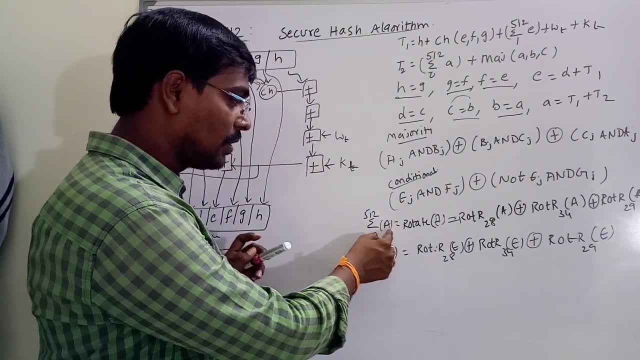 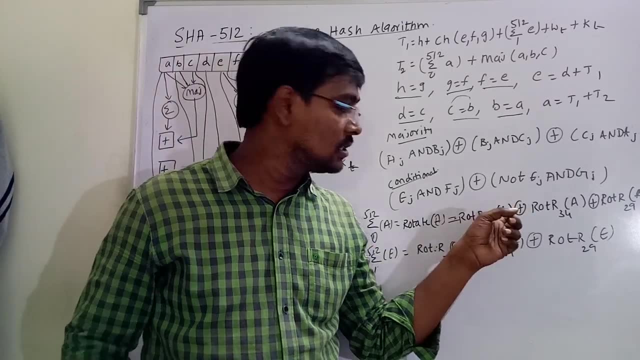 For example, sigma 0 to 5, whole of N is rotate of A. Rotate of N is rotate 28 of A. That is on 8 is rotated by 28 bits With 34 to 29.. This is on 8..